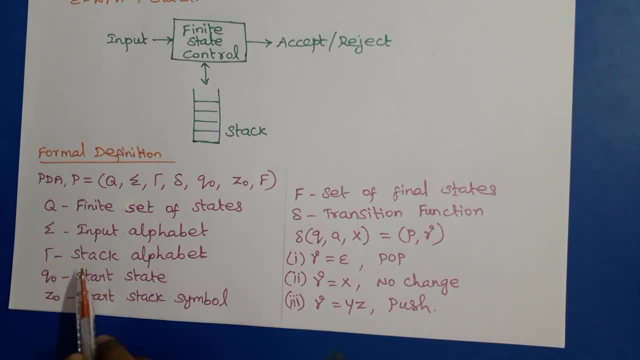 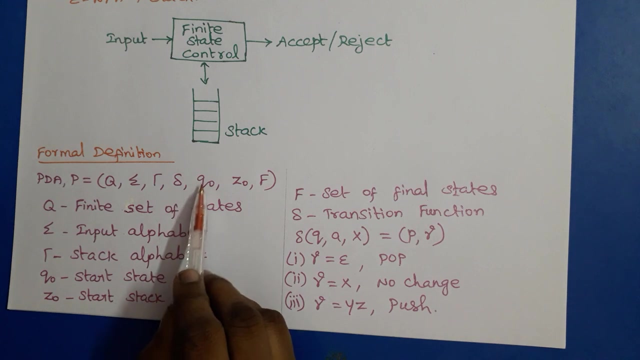 And gamma is a stack alphabet, that is, a set of stack symbols. in the stack symbols We will push the some terminals as well as variables, So these are called as stack symbols. So gamma represents stack alphabet, Then delta- we will see it later- Q naught. Q naught is a start state of the finite start state of the PDA, Then Z naught is a starting symbol of the stack. Okay, So initially stack will contain: 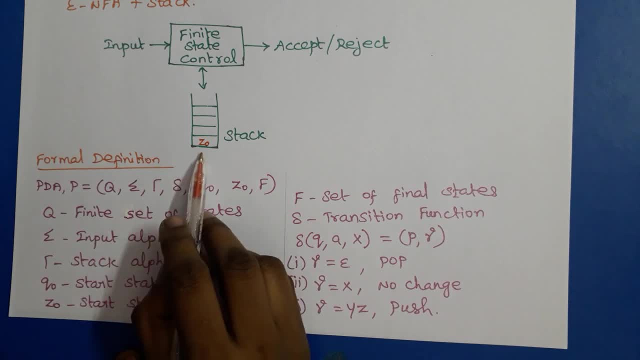 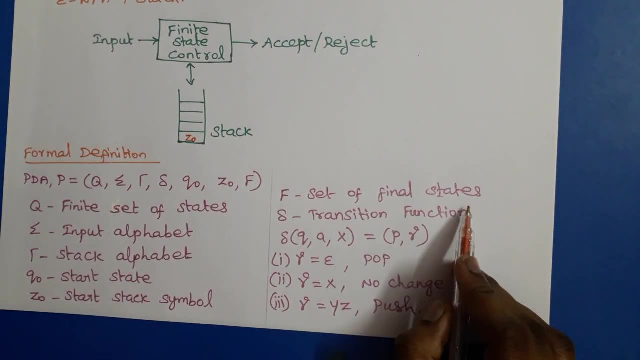 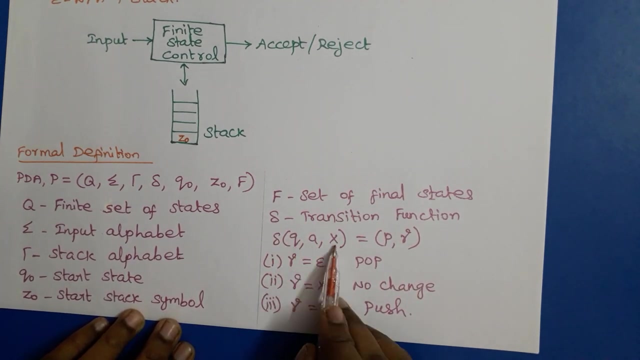 Z naught in the bottom bottom of the stack. Okay, So this is the stack starting stack symbol and F is a set of final states or accepting states and delta. delta is a transition function of a PDA. It takes three arguments as input: Q A, X, So delta of Q, comma A, comma X, where Q represents present state, So current state of the finite control. current state of the finite control. 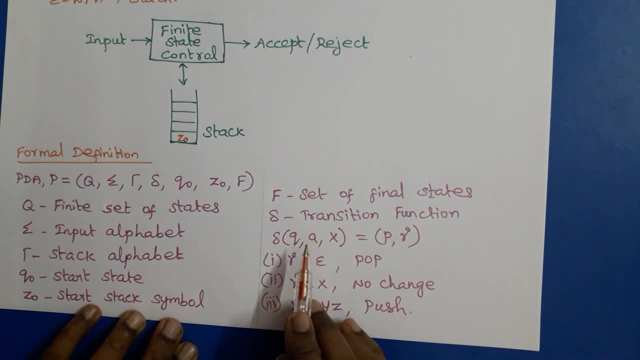 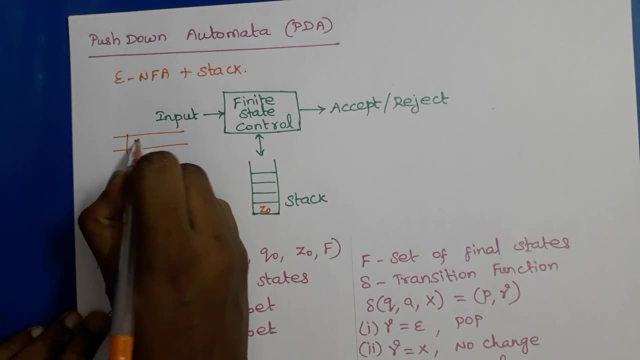 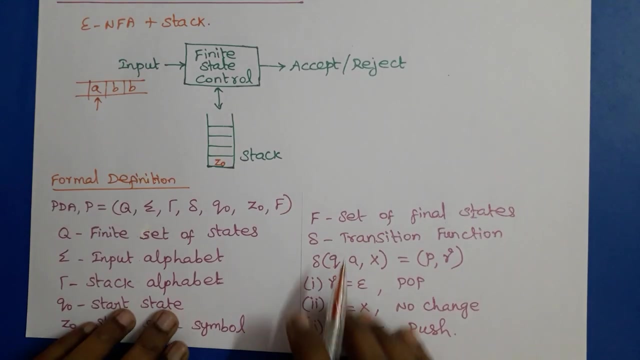 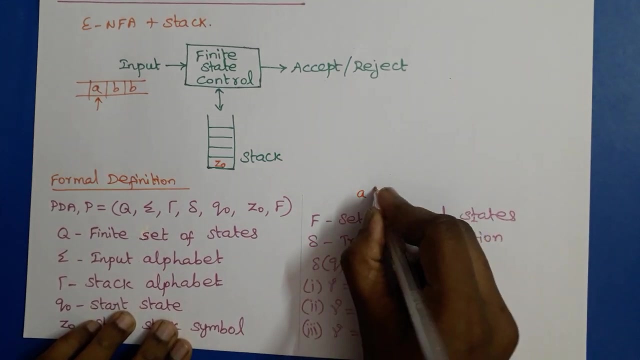 PDA is represented by Q and A. A is a input symbol on the input string. So for example, if the input string has some input string- A, B, B- and initially the finite control is pointing to A, means that symbol is A and it may be epsilon also. So A is a symbol in sigma or A equals epsilon. 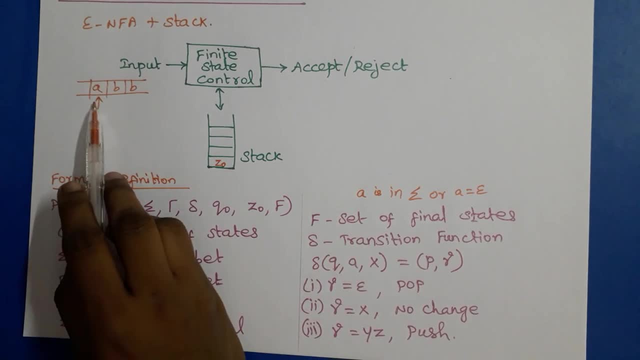 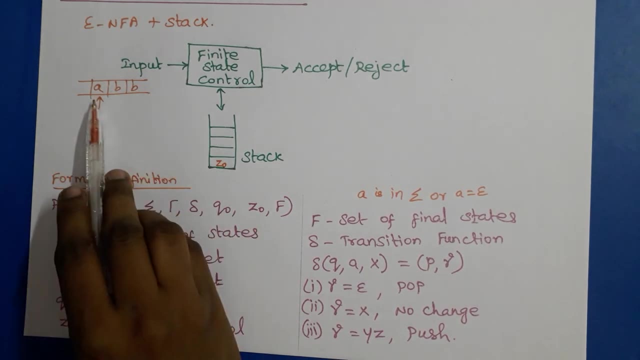 So if A is considered as a input symbol, then the thing is that input symbol is consumed from the input string. So in the next step we will read the next input symbol. But if epsilon is considered as a input symbol, the thing is, without considering the input symbol, we can change our state to next state. So input the input pointer will not advance to the next input symbol. So this Q, Q means current state. 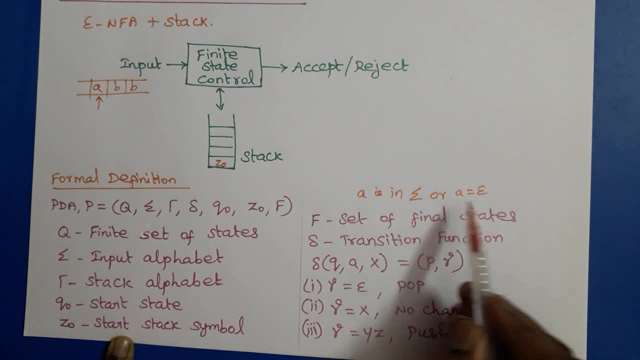 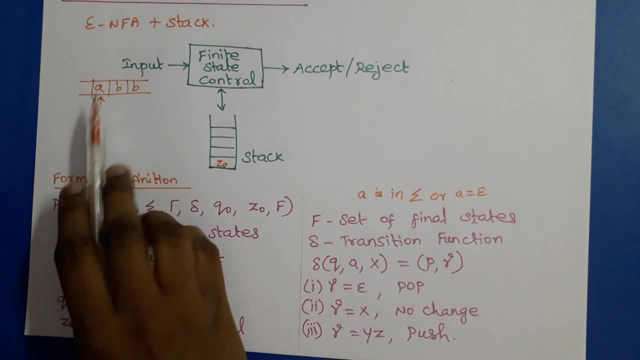 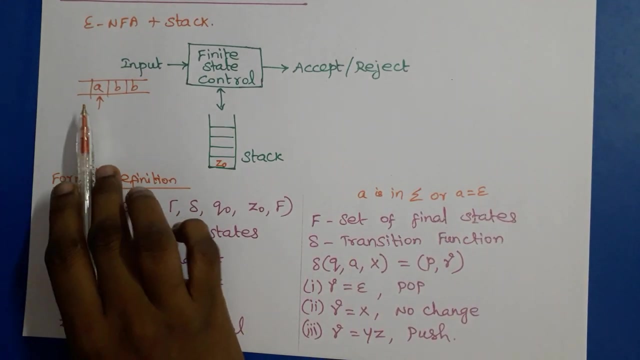 And A is a current input symbol. It may be epsilon also. If the input symbol in sigma is considered, then in the next step we need to the input pointer should point to the next input symbol. The thing is input symbol is consumed from the input string But epsilon is considered as a input. Here epsilon is given, then the thing is we should not consume the input symbol. 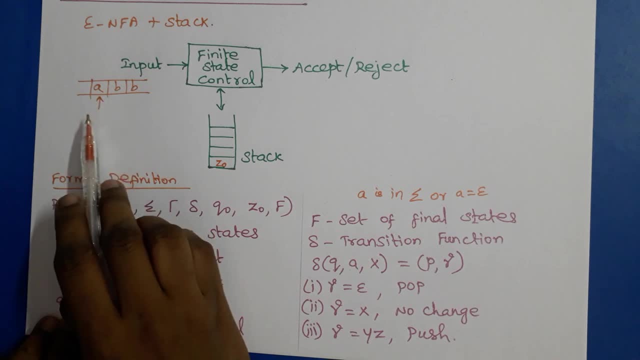 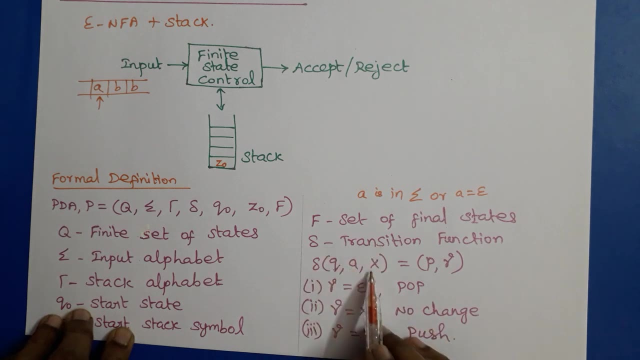 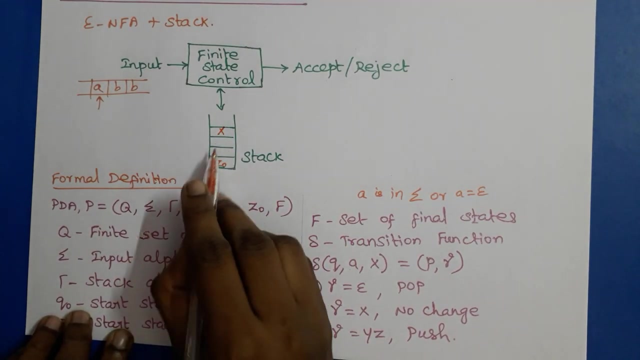 In the next step. also, we need to point the. we have to read the same input symbol in the next step. then the third symbol in the transition function represents x. that is top of the stack. so assume that now the top of the stack is x. it may. 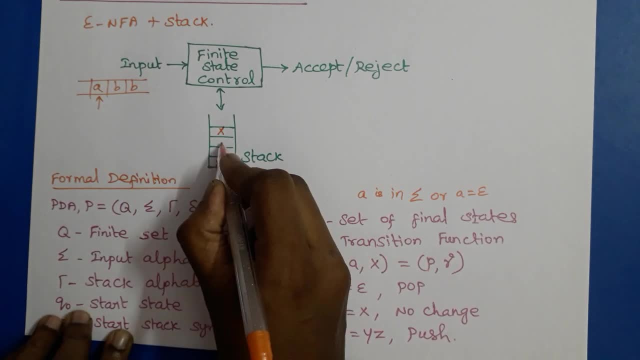 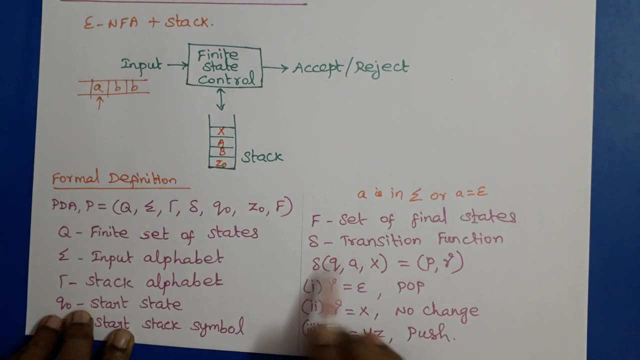 be preceded by any any symbols, for example here a, b, any any symbols may be there, but x means top of the stack and in one move, in one move the pda can change its state to the next state, p. okay, so it takes three arguments as input: q, comma, a, comma, x, that is current state of the pda and current. 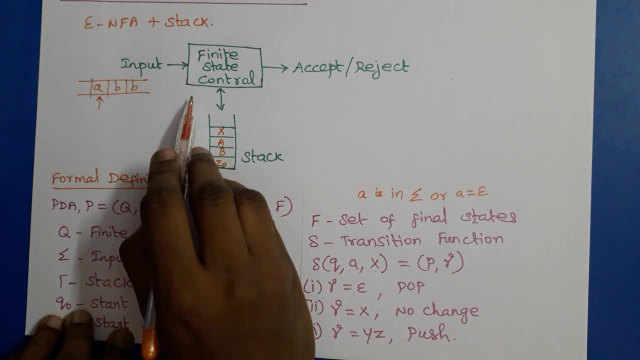 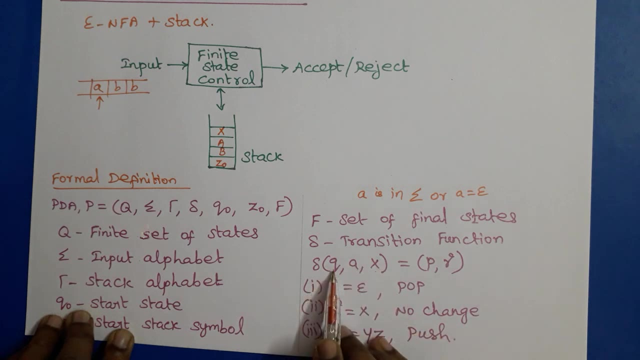 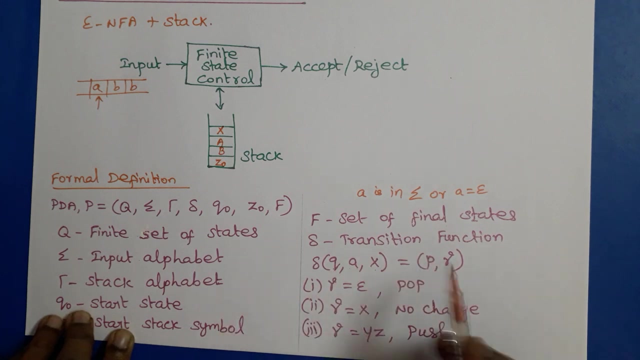 input symbol and top of the stack, state of the pda input symbol and top of the stack. and it performs three operation, three things. one is it changes its state to next state p. so sometimes it may be same as a previous state. here also we may. it may remain in the same state. so in that case we need 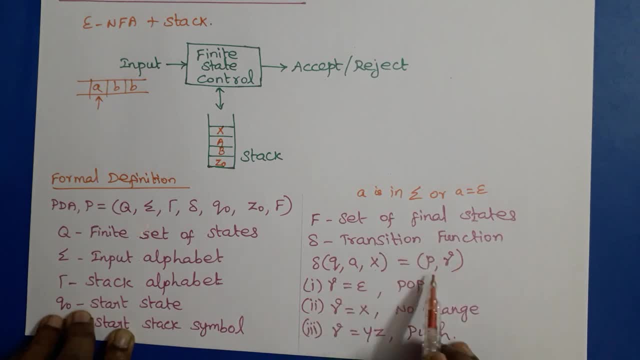 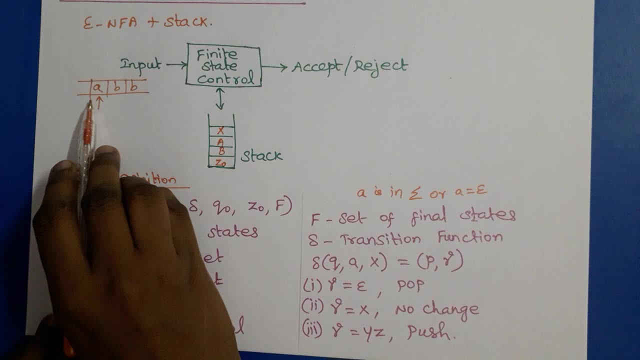 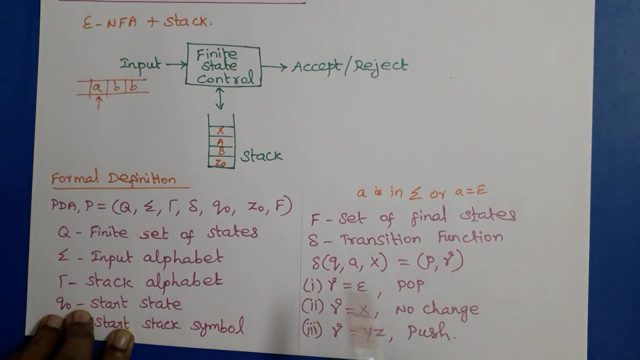 to write q here instead of p. so now in here it changes its state to p. then if a is written here, then a is consumed from the input string. epsilon is written, then it should not consume anything. the thing is without reading input. it can change its state to p and x. the top of the stack is x. 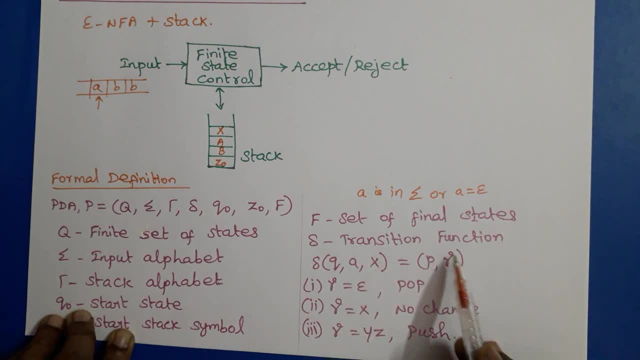 is replaced by x string. gamma- this is the gamma- is a string and here there are three possibilities. if gamma is epsilon, then pop of the stack is performed right, because x the top of the stack. assume that the top of the stack is x means it is replaced by epsilon. it is replaced by epsilon. epsilon means: 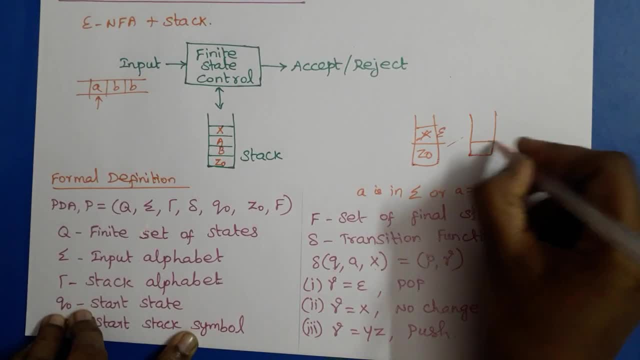 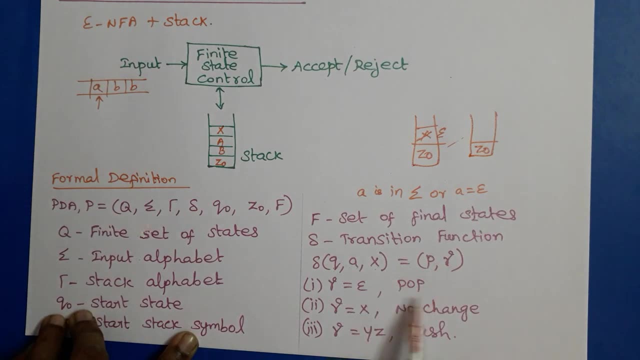 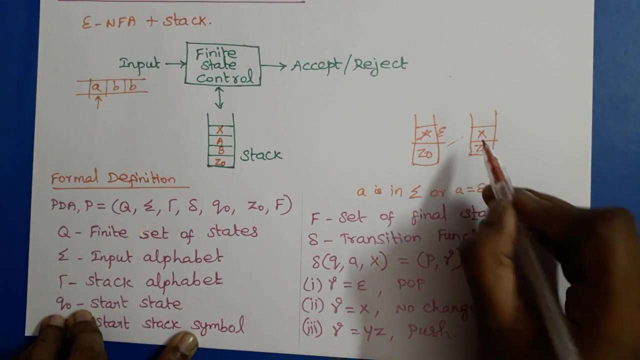 pop of the stack is performed. we should not write anything right. x is replaced by epsilon. the thing is, x is popped from the stack. if gamma is equal to x means then this gamma, that is x, replaces x on top of the stack. so if top of the stack is x, then this x is replaced by same x. 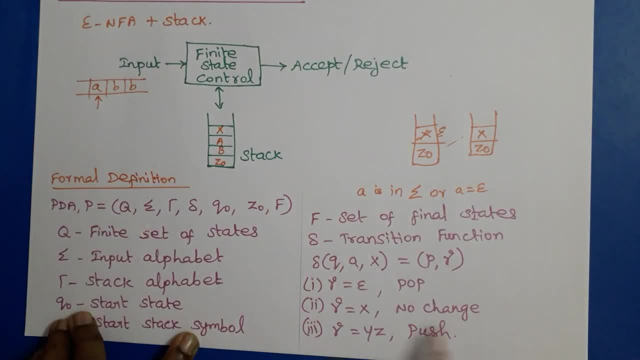 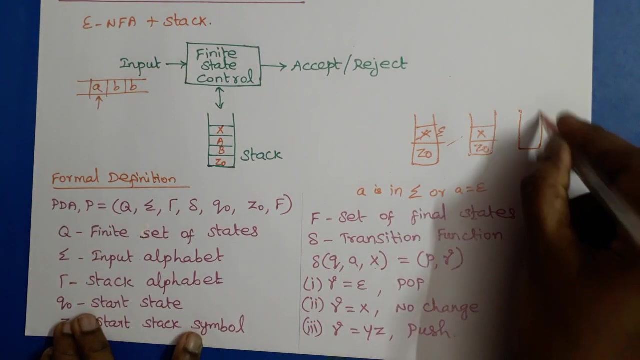 so what happened here? no change in stack, that operation is performed. no change operation is performed here. but if gamma has some string of symbols, that is, if gamma is equal to y, z, then push operation is performed. that is this: z replaces x on top of the stack, then y is pushed onto the stack. that means x is replaced by z. right end of. 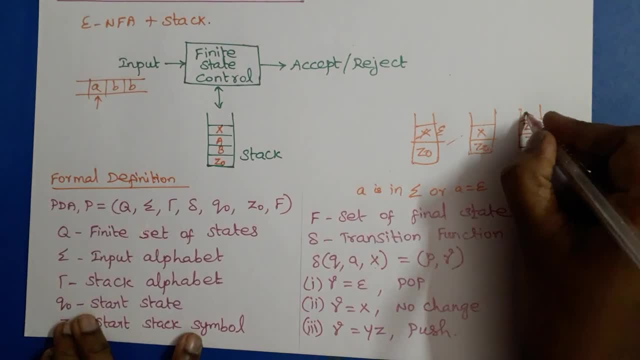 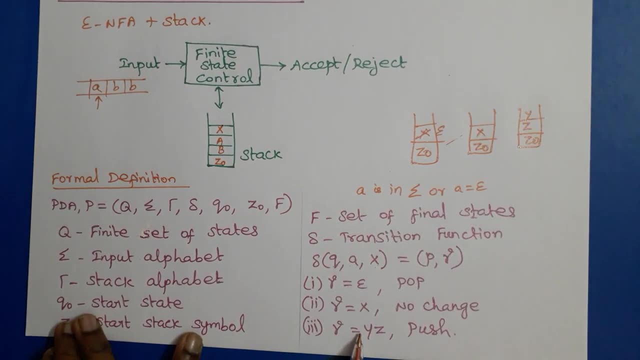 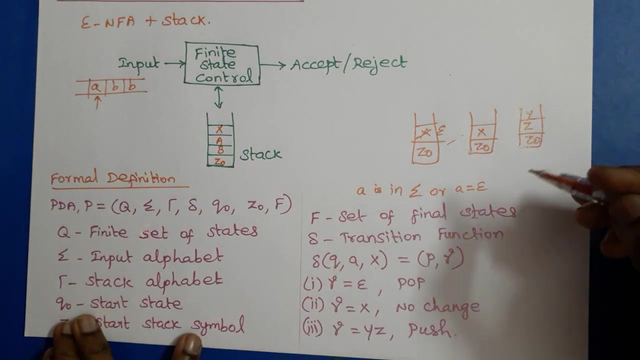 string, then the next symbol will be pushed onto the stack. suppose it has another symbol here, for example w, w will be. will also be pushed onto the stack. so left end of the string maybe will be in the top of the stack, right end will be in the bottom. after above the z naught. 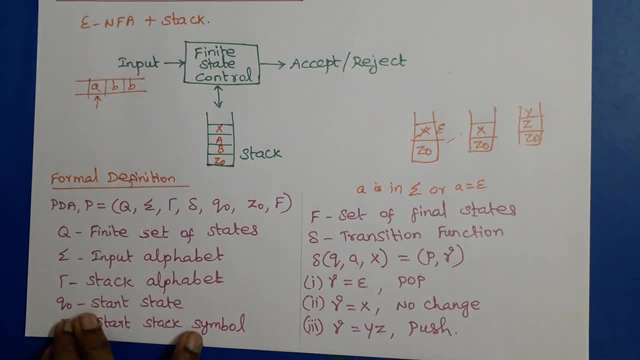 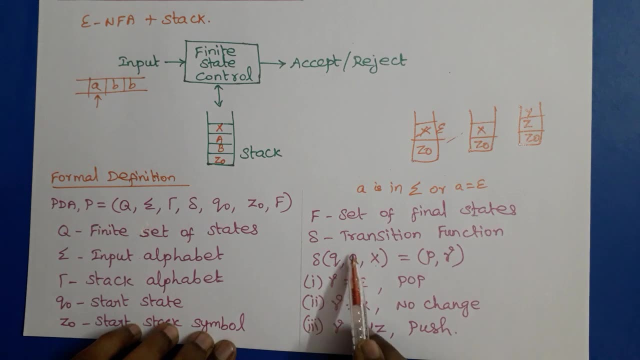 right end will be there. okay, so in one move the pda changes its state from q to p. and if the input symbol is a, it any symbol in sigma, it will be consumed. or if the input symbol is a, it will be. if it is a epsilon, then it is not consumed. input symbol is not consumed. and this is the second. 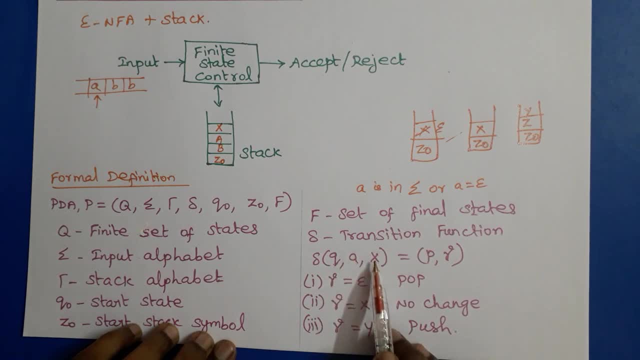 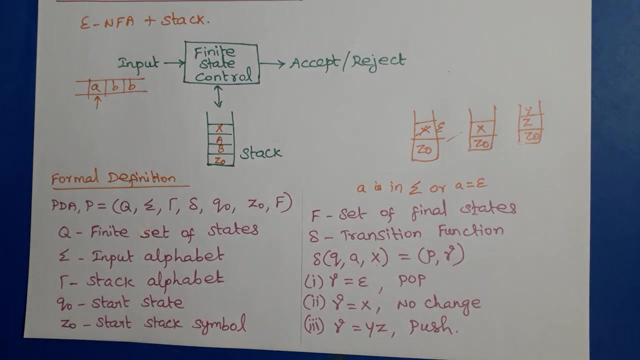 operation. then the third one is top of the stack: x is replaced by the gamma. if gamma is epsilon, pop operation is performed. if gamma is same as the symbol, no change operation. if gamma is some other set of symbols, then push operation is performed. now we will see an example. 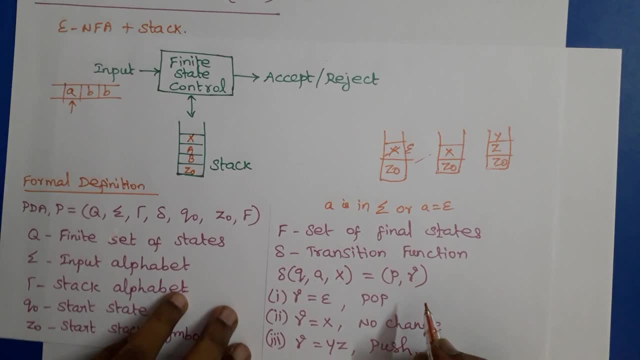 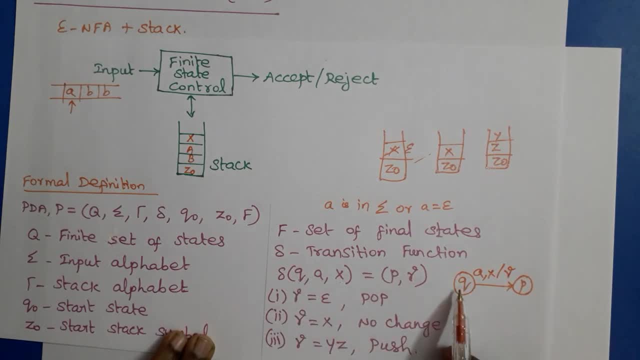 slash gamma. okay, so the thing is: delta of q comma, a comma x equals p comma gamma. that is um current status. q current input symbol is a top of the stack is x and the next state is p and the um string that replaces x on top of the 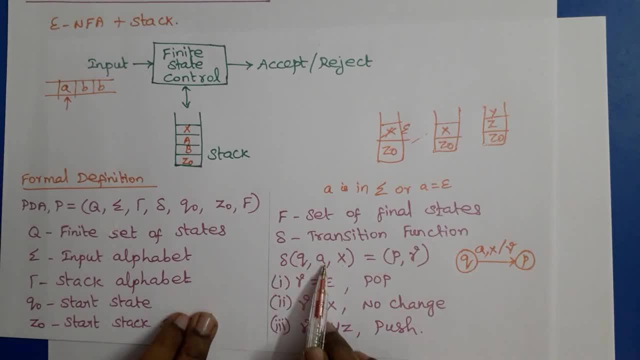 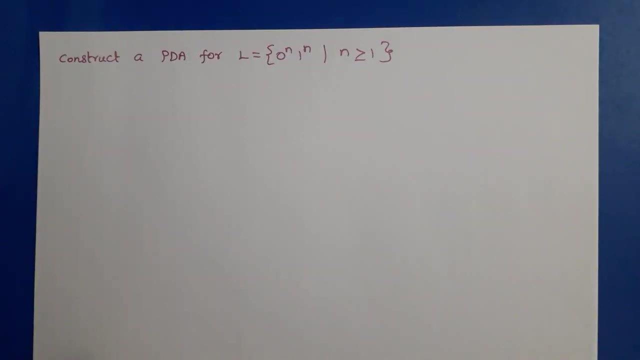 stack is gamma. and one more thing: in the non deterministic, finite state automata, delta of q comma, a, comma, x contain contains only one pair. but in non-deterministic, finite automata it may contain some, any number of pairs. okay, because it is non-deterministic, now we can construct a pda. 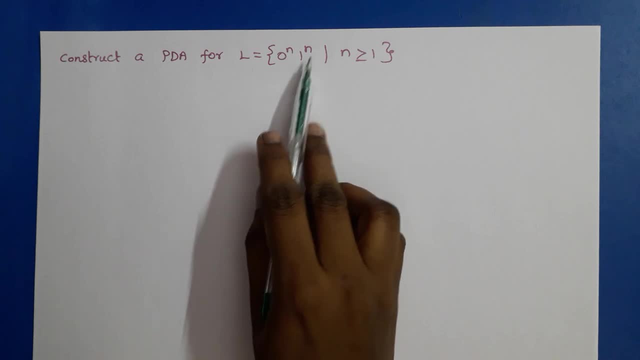 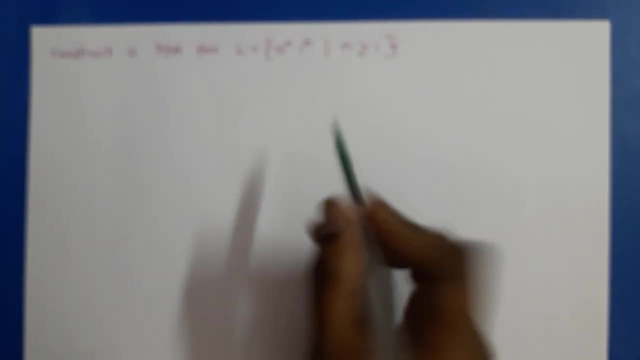 for language l is equal to p comma a comma x equal to p comma a comma x. equal to p comma a comma x. equal to 0 to the power n, 1 to the power n, such that n is greater than or equal to 1. so here the set of strings accepted by this language um are: 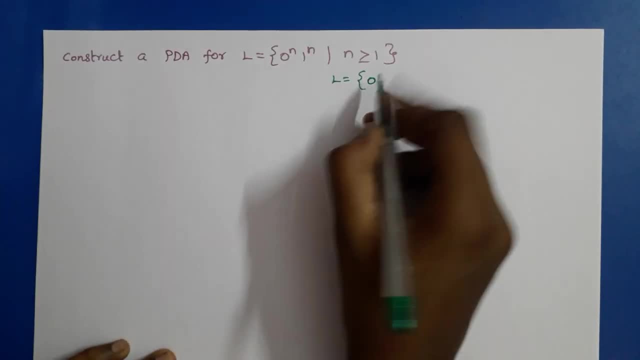 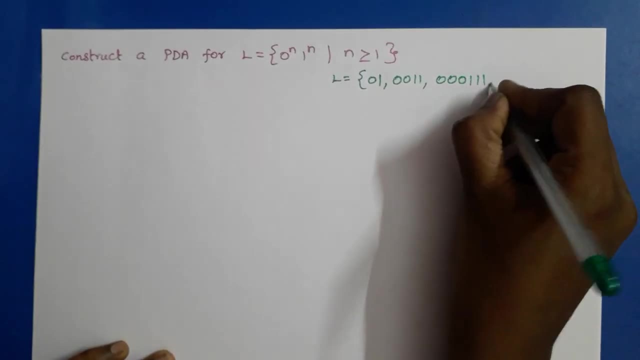 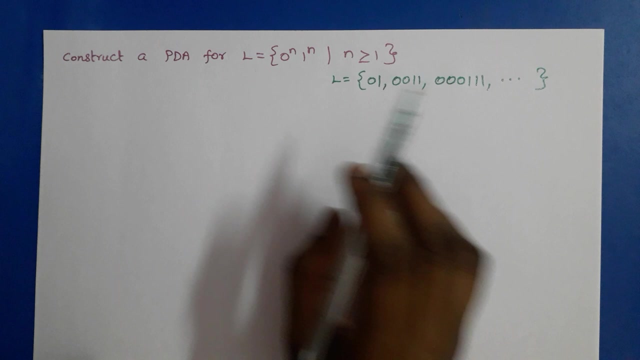 single 0, 1. if n is 2, then two zeros, two ones, three zeros, three ones, etc. right, so n number of zeros, followed by n number of ones means that string must be accepted by our pda, otherwise it is a incorrect input string. so now we have to construct a pda for language. l is equal to p comma, a comma x. 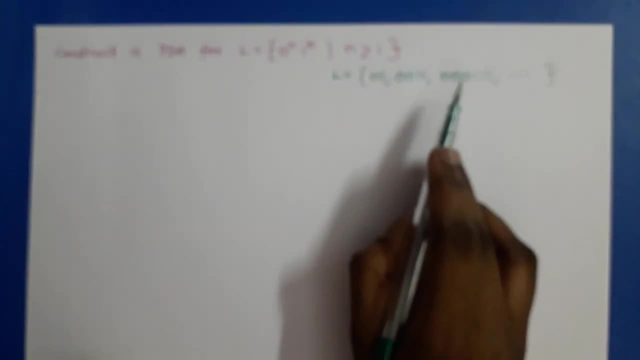 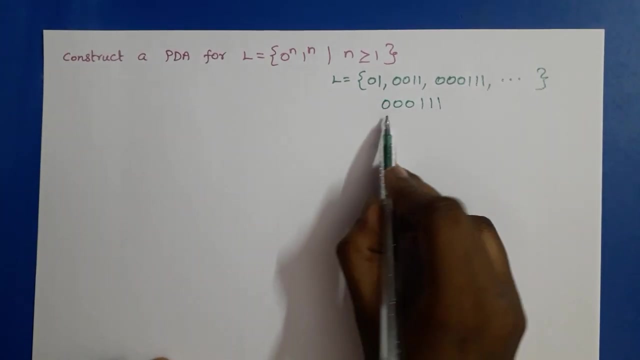 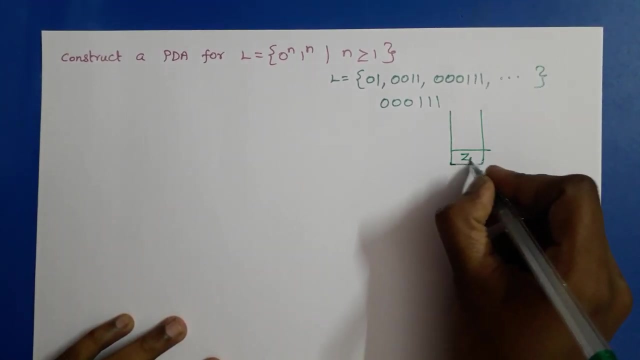 so we have to construct a pda for accepting these type of strings. so the concept is, for example: consider triple zero, triple one, so for first we will see n number of zeros. right, so we have to push all zeros onto the stack. so whenever we read zero, that must be pushed onto the stack. 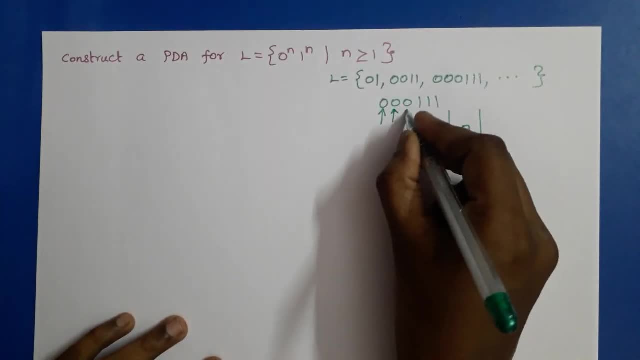 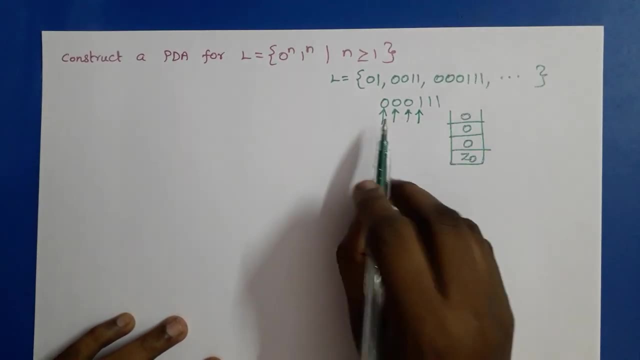 the next symbol is also zero. third symbol is also zero. so that should also be pushed onto the stack. so we have to push all zeros onto the stack. so whenever we read zero, the stack. next we will see n number of ones. right after pushing n number of zeros onto the stack, we 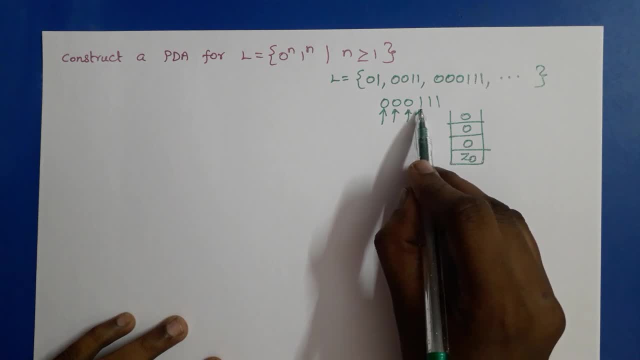 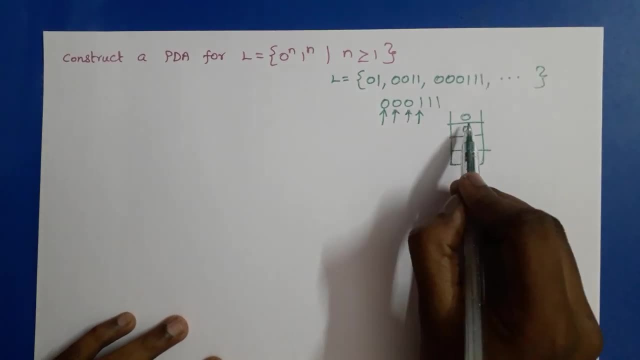 will start reading number of ones so that for each one we have to match with the zero. each one is matched with one zero and pop should be performed. so first we will read first one, then that is matched with the top of the stack. that means for each one we have to pop. 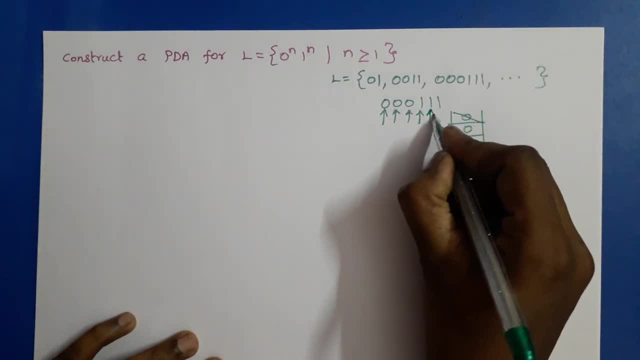 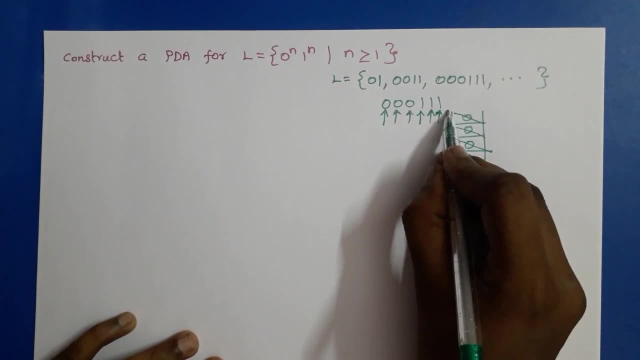 one zero from the stack. then next input is one. again we need to perform pop operation. next input is one. again we need to perform pop operation. now the input symbol is input symbols are fully consumed, so the assume that the next input is next symbol is epsilon. so when we read epsilon, 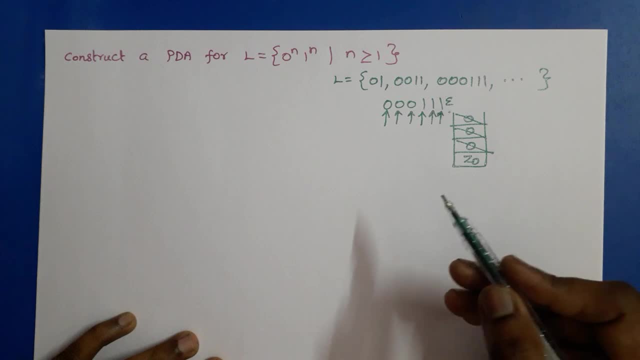 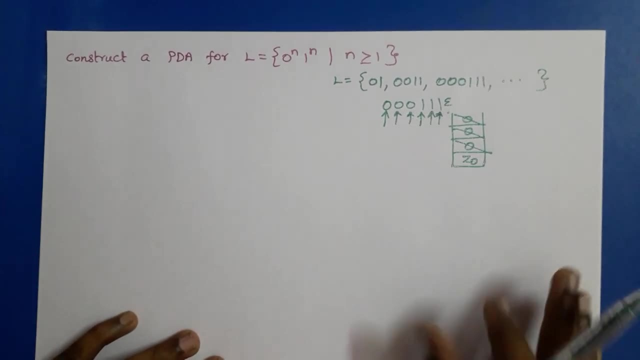 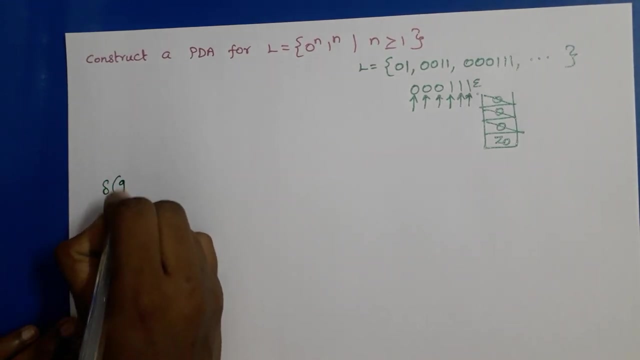 the top of the stack is z naught means then we can accept the input string because it has n number of zeros followed by n number of ones. so this is a concept. so we have to perform pop operation. now we will construct the PDA for this problem. so delta q naught comma, assume that q naught is a. 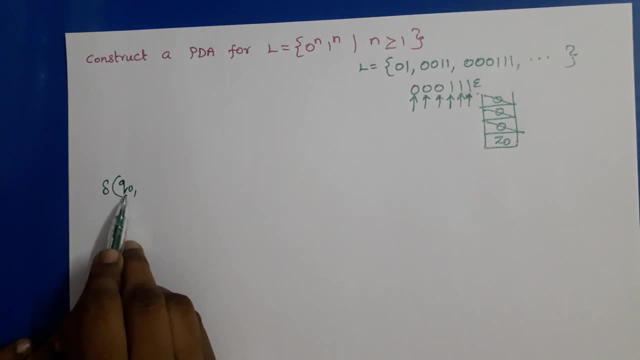 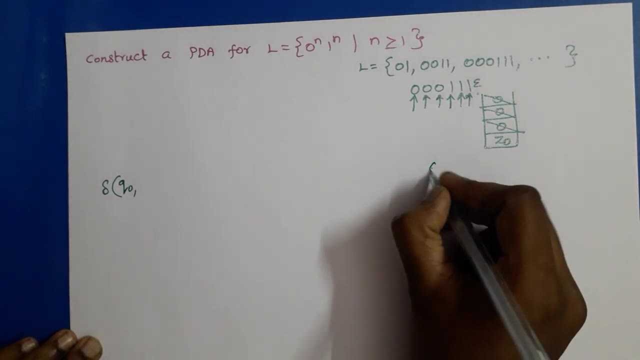 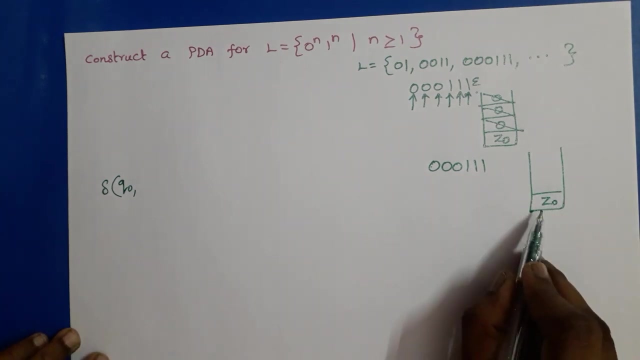 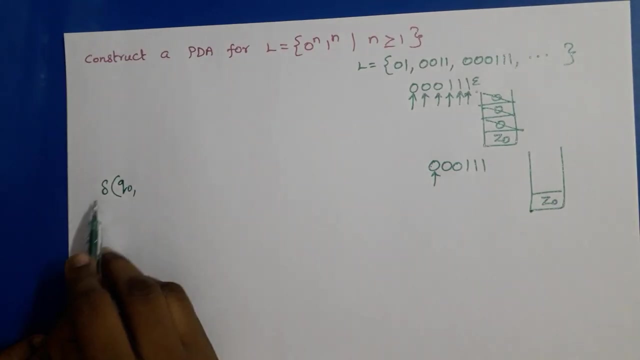 current state, start state of our PDA. so q naught is a current state and next input symbol is: assume that this is our input string and z naught is on stack initially. so the first input symbol is zero. first we will read some number of zeros right. so delta of q naught is a current state, zero. 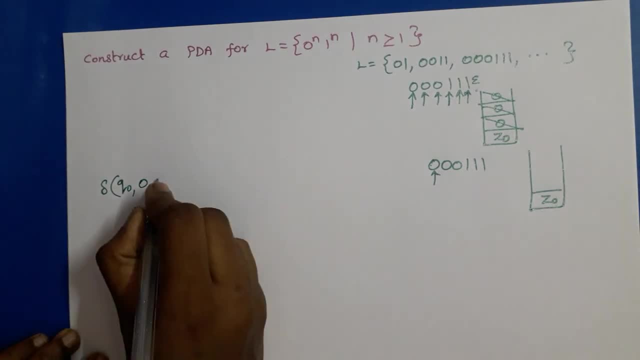 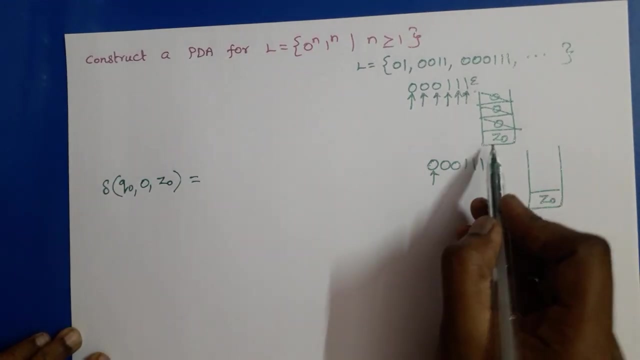 is the input symbol and z naught is a top of the stack. so here we need to write current state, current input symbol and top of the stack. so if zero is a input symbol we have to perform, it should be inserted into the stack. right push operation should be performed so that we should 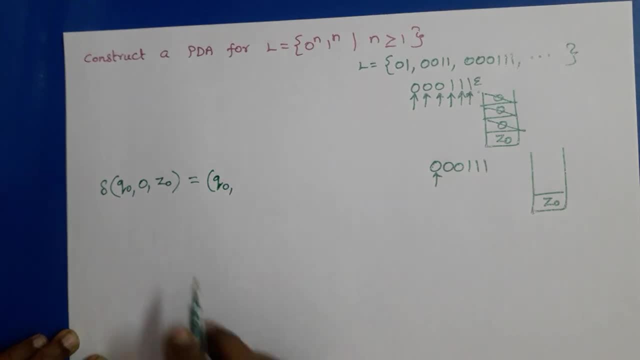 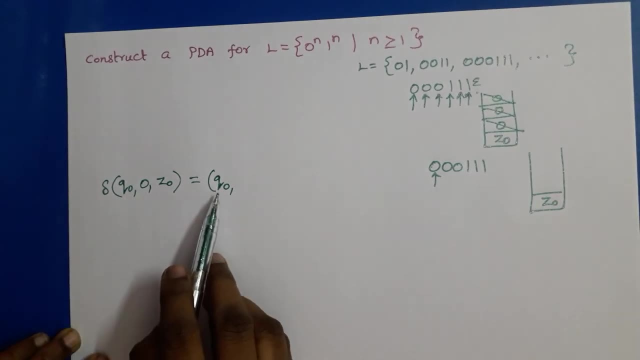 remind the input symbol to be inserted into the stack, so that we should remind the input symbol in the same state- q naught, because we are going to insert all zeros onto the stack. it is a repeated step, so we should still remain in the same state- q, naught, and zero must be pushed onto the stack. 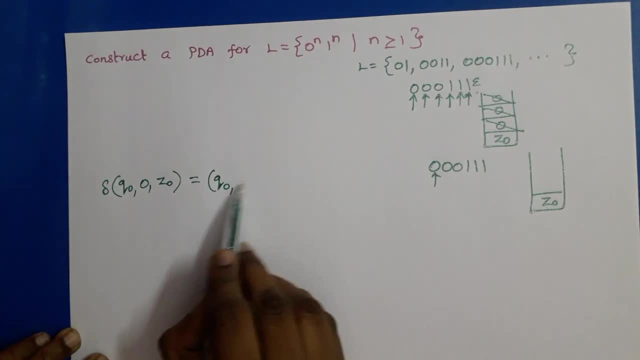 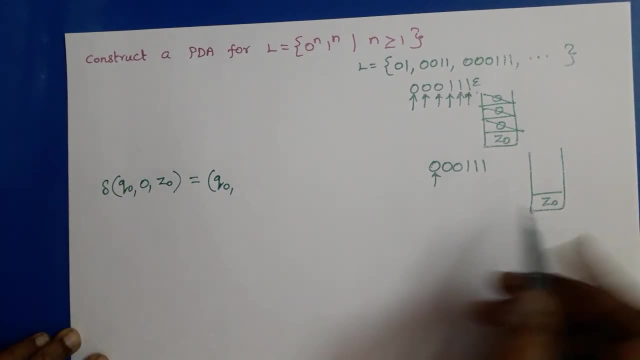 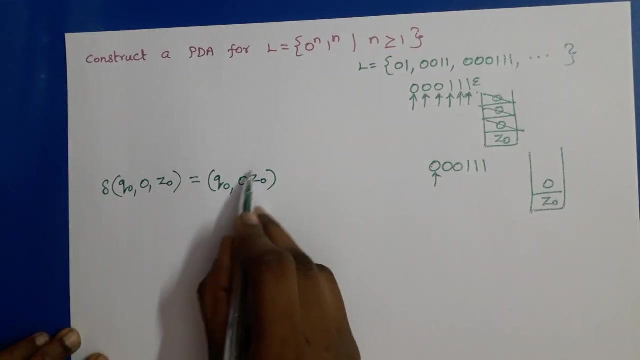 so the thing is: whatever written here that will replace z naught top of the stack, so that if you want to push zero, then here you need to write zero, zero, z naught. okay, because always the right end of this string will replace top of the stack. 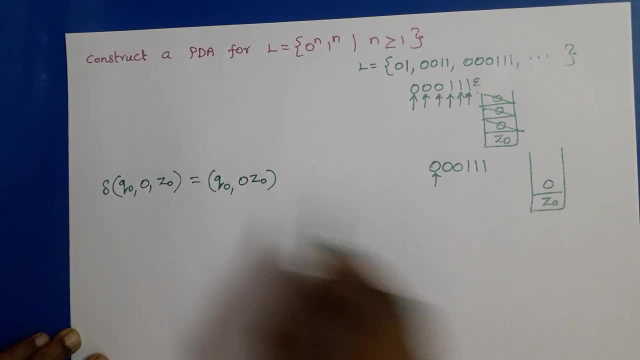 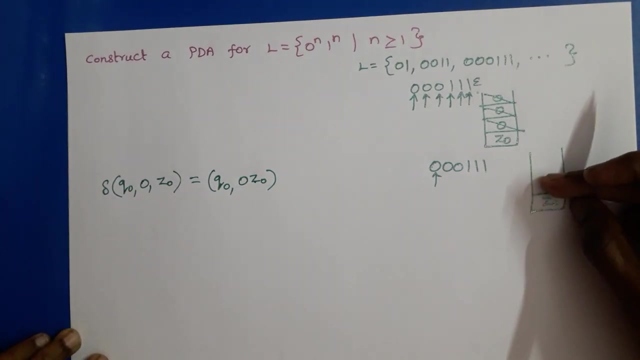 so z naught replaces z naught and zero is pushed onto the stack right. so when we perform push operation, just combine these two symbols and write the thing is z naught. this symbol will replace z naught on top of the stack. z naught is there in the at the beginning, so z naught replaces 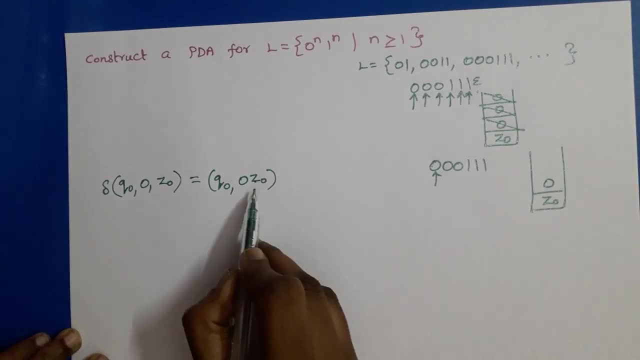 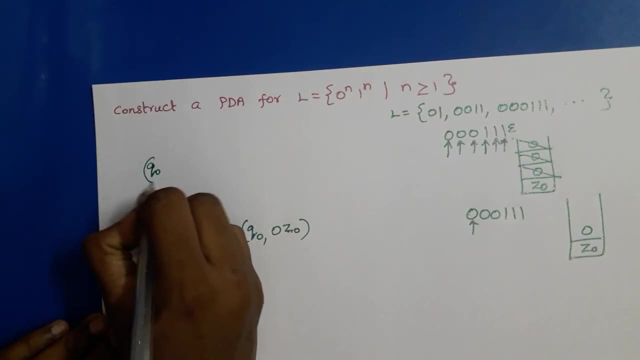 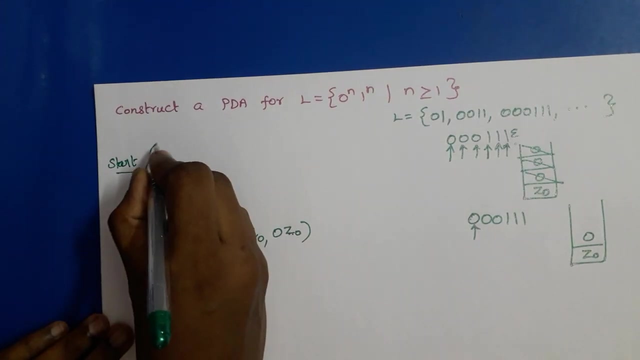 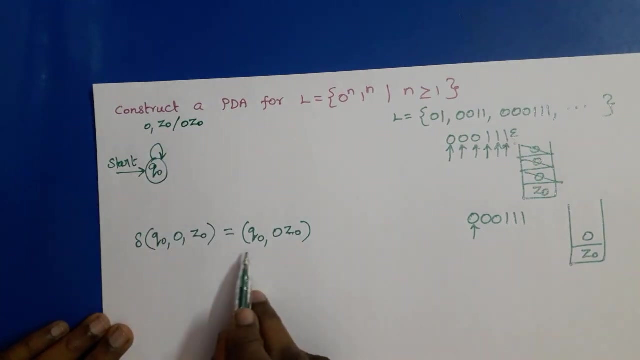 z naught and zero is pushed onto the stack. z naught replaces z naught and zero is pushed onto the stack. so when we draw the transition diagram for pda, start, q naught is a start state and from q- naught to q naught. so, yes, self loop and that is labelled by zero comma z naught, zero comma z naught. forward slash: zero z naught. 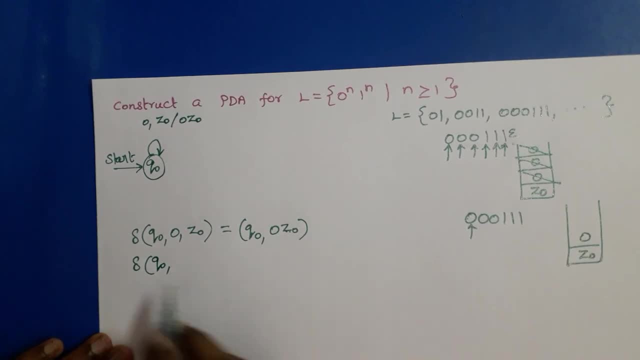 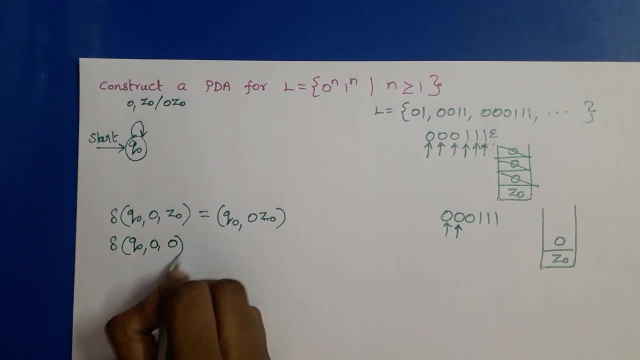 Now we are in state Q naught, So Q naught. next, input symbol is again 0 and now top of the stack is 0, right. So if the input symbol is 0, again, we need to perform push operation. 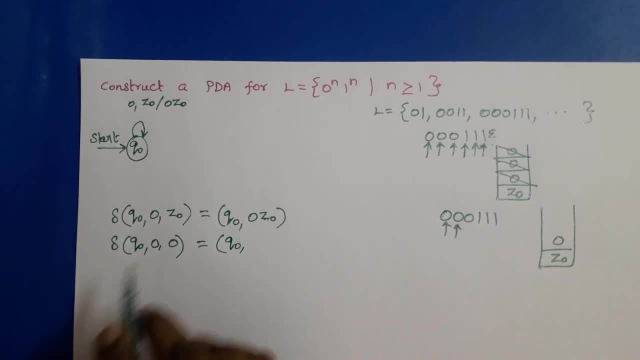 So we should remain in the same state: Q naught, and again we need to perform push operation. So 1, 0 we have to write for replacing top of the stack. This 0 is replaced by this 0. So then 1 more 0 should be pushed onto the stack right. 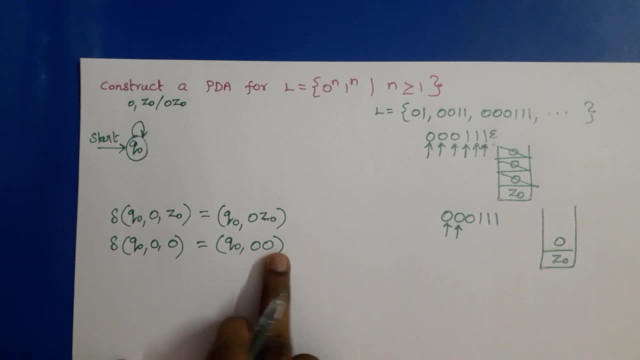 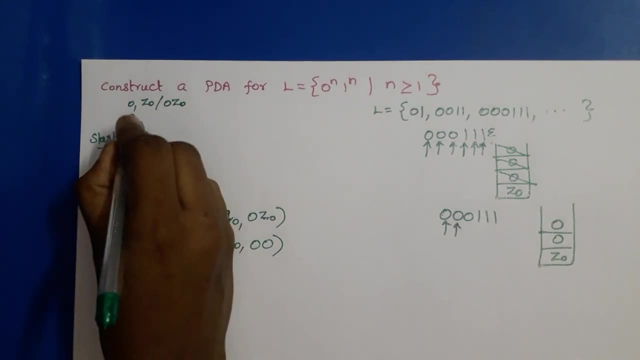 So we have to write 0: 0 here. So Q naught comma 0: 0.. So 0 is pushed onto the stack. So here also we have to write 0, comma 0, slash 0: 0.. 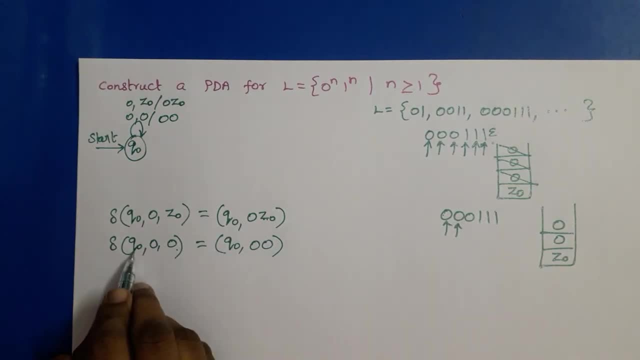 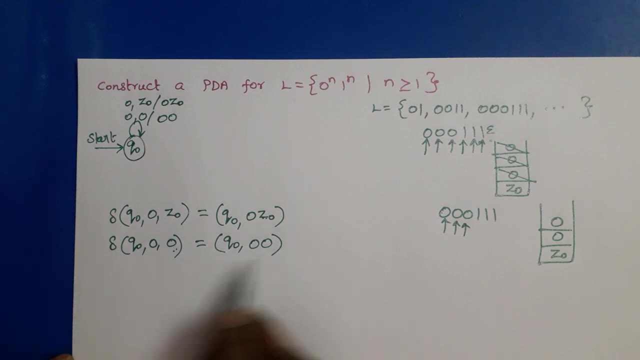 So now the current state is Q naught. Current input symbol is 0.. Top of the stack is 0. So there is no need to write a new transition. This is the transition for that. Q naught is a current state. 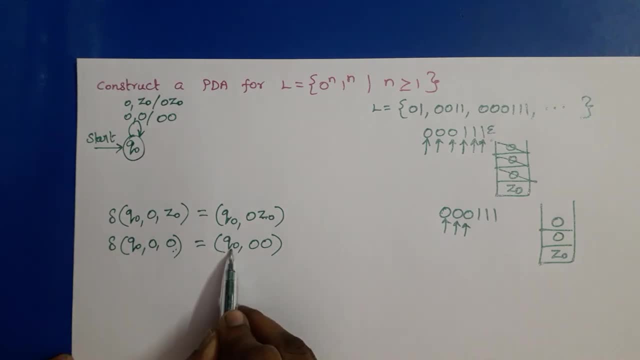 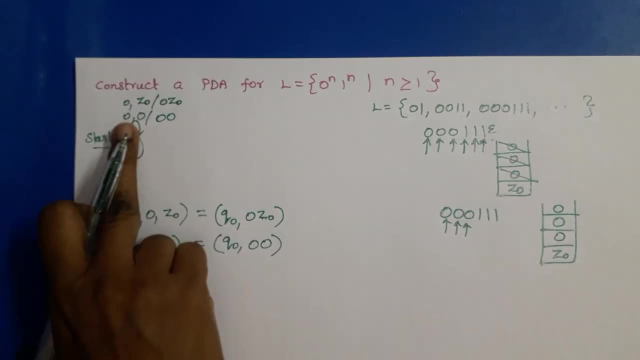 Current input: 0.. Top of the stack is 0. So we will remain in the same state: Q naught and 0 is pushed onto the stack. So this operation is performed and 0 will be pushed onto the stack. So there is no need to write it in the transition diagram also. 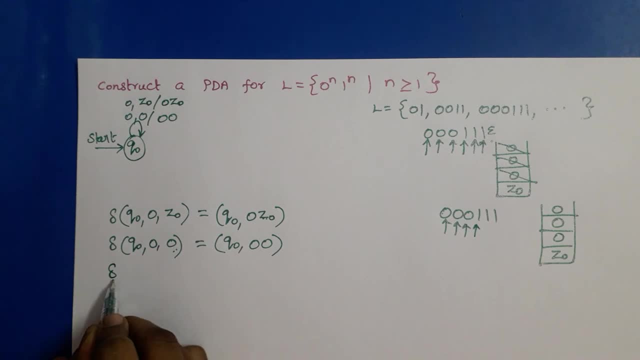 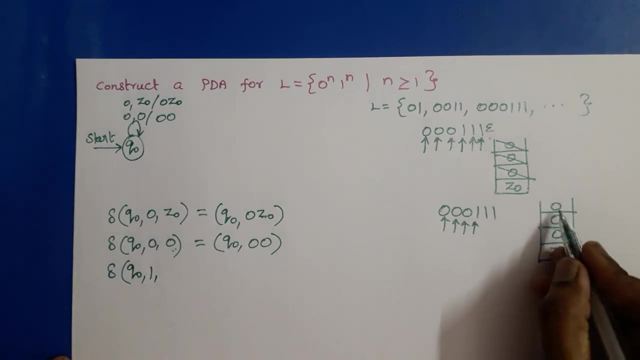 Next input is 1.. So we have to write a new transition. So delta Q naught is a current state, 1 is an input symbol and top of the stack is 0. Means we have to go to the next state. 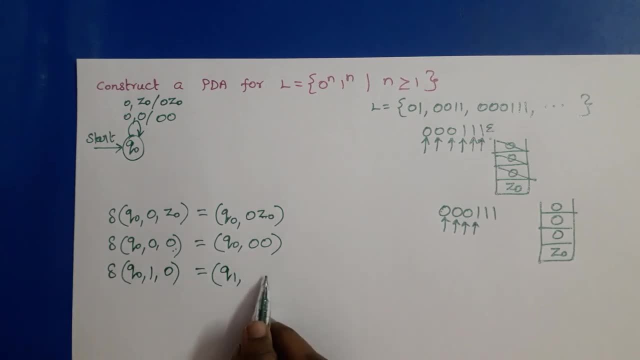 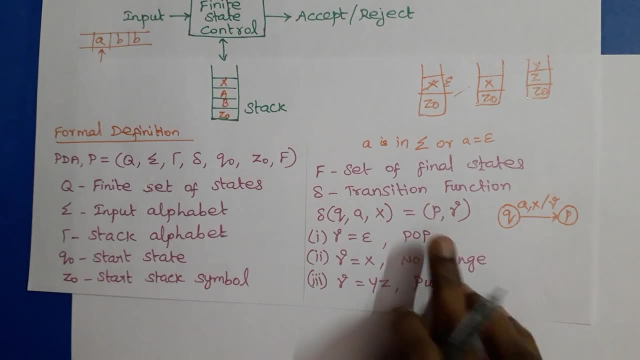 Q1 and pop operation must be performed For each 1,. 1, 0 must be popped from the stack. So to represent pop operation, we have to write epsilon here. If you want to represent no change operation, we need to write the same symbol, X, here. 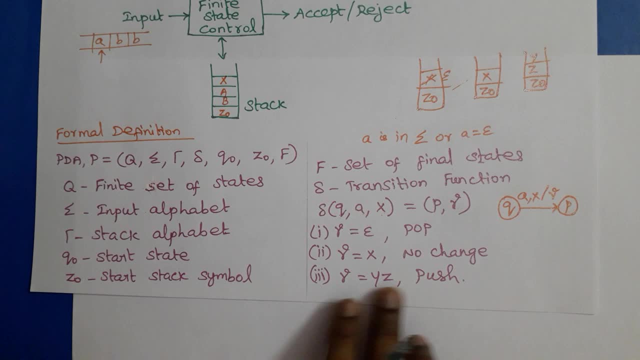 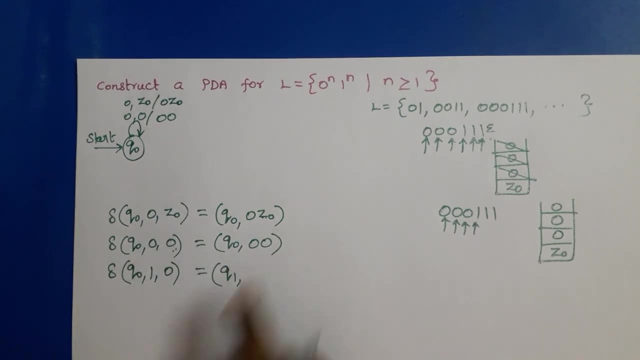 If you want to perform push, then we have to write sequence of symbols here. So for push operation we have to write 0, Z naught here, 0, 0 here. But for pop operation we need to write 0- Z, naught here. 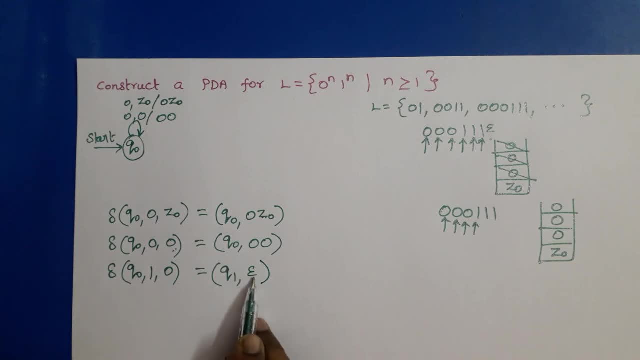 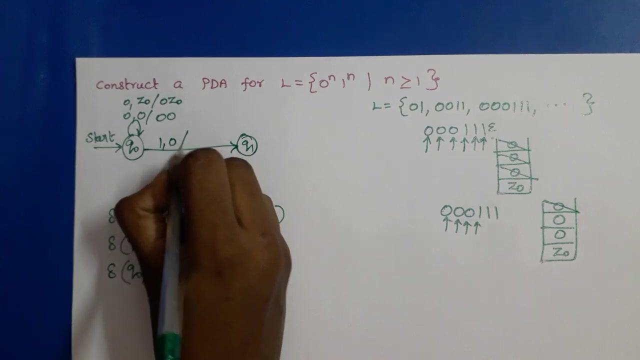 So we have to write epsilon. So the meaning is this: epsilon replaces 0. So 0 is removed. The meaning is: 0 is removed. And from Q naught to Q1, draw an edge. That edge must be labeled by 1 comma. 0 slash epsilon. 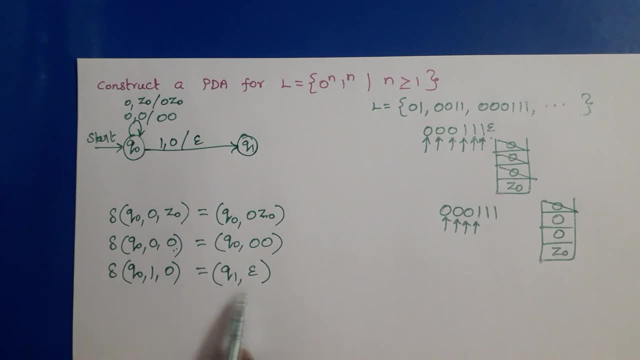 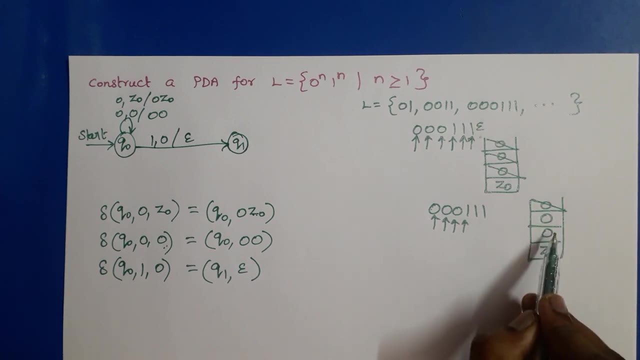 So from Q naught to Q1.. So this operation, this transition function, is used for popping 1 symbol, 1, 0 from the stack. So to repeatedly pop All the symbols, all the 0s, we have to write a recursive definition. 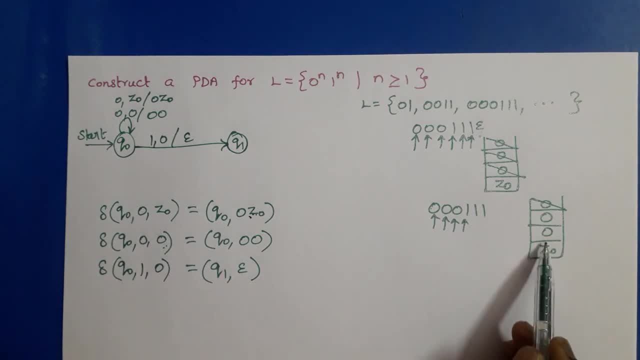 Okay, So in the first step we have pushed 1: 0 onto the stack By following the second. one is second one only is used for performing pushing all 0s onto the stack. Similarly, the third transition function will pop 1: 0.. 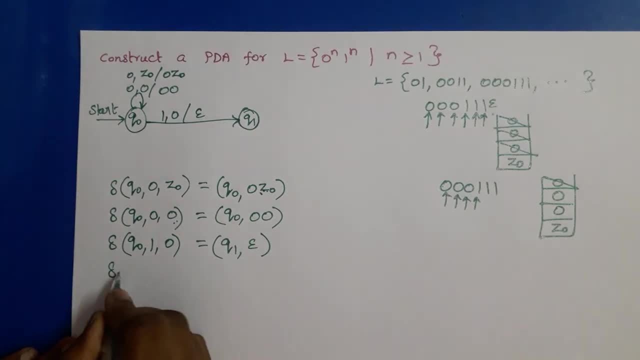 To pop all the remaining 0s we have to write the recursive definition. So Q1 is a current state. Next input is 1.. Top of the stack is 0.. Now this 0 is popped, So top of the stack is 0.. 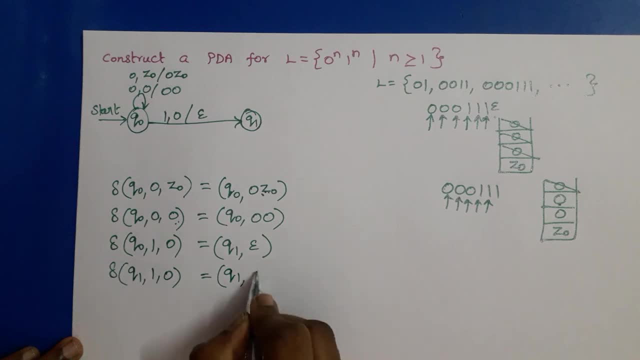 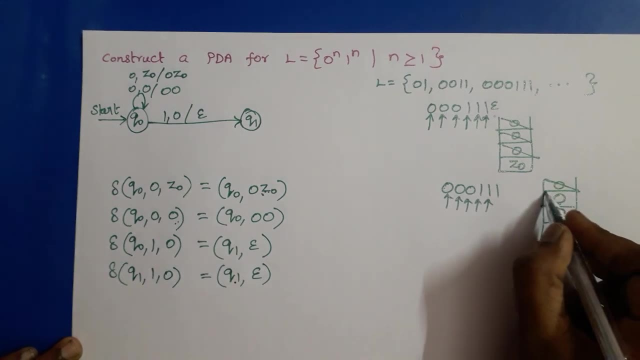 Means we have to remain in the same state. Q1 and pop 0 should be performed. Okay State remains in Q1, but 0 is replaced by epsilon. The meaning is it is also popped. So from Q1 to Q1, draw an edge. 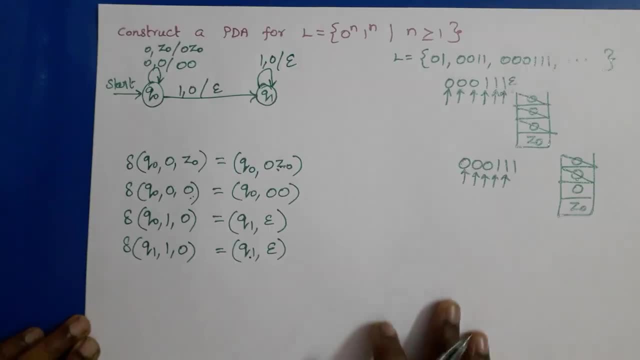 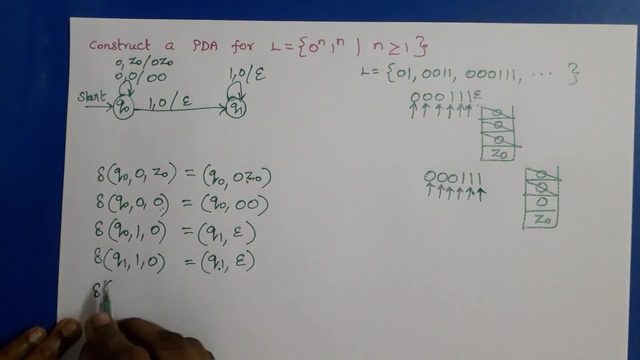 That edge is labeled by 1 comma 0 bar epsilon. Then again, Now we are in state Q1.. Next input is 1.. So Q1 and the next input is 1.. Top of the stack is 0.. 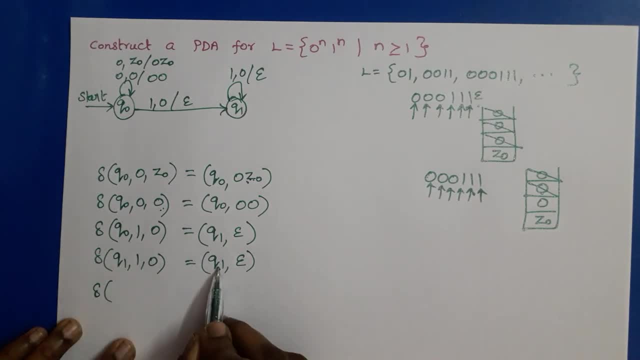 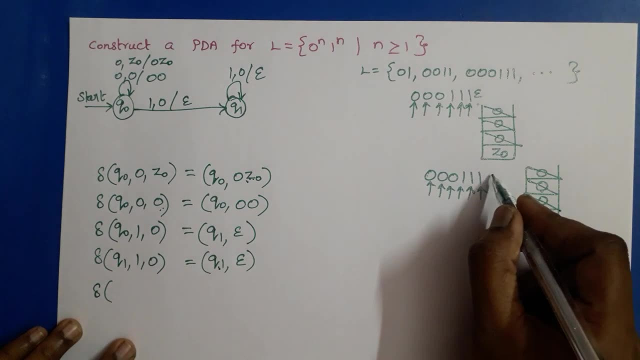 So the same transition function is performed. So the next state is Q1 and 0 is popped. So there is no need to write a new transition. This is also popped from the stack. Now the meaning is: epsilon is here. 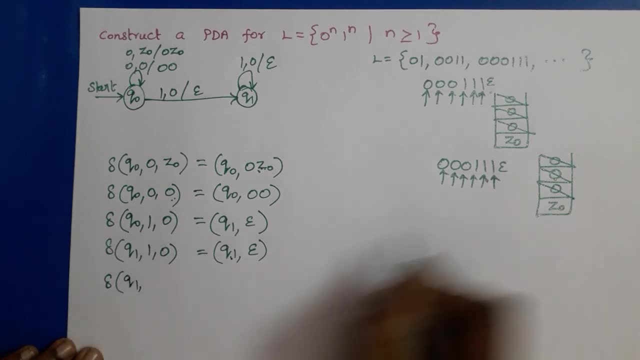 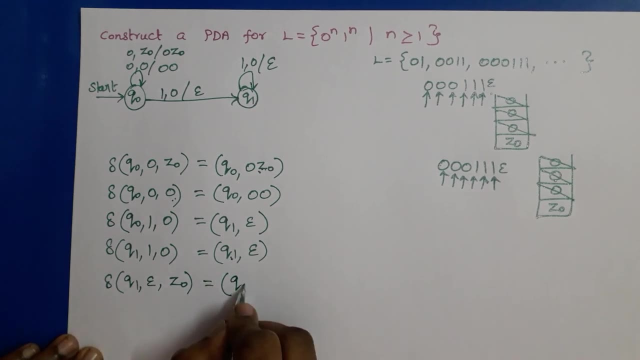 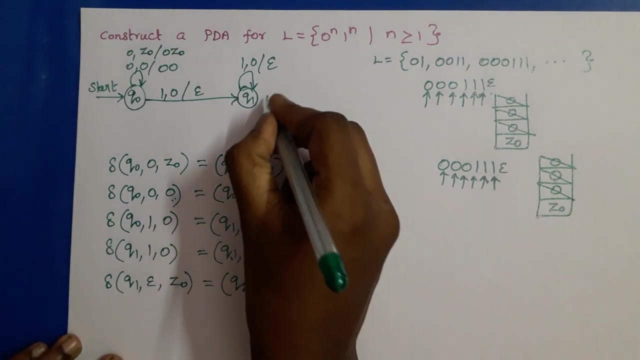 So Q1 is a current state. Epsilon is the input. Top of the stack is Z naught Means we have to go to the final state, Q2 and Z naught. No change in Z naught. So from Q1 to Q2,. 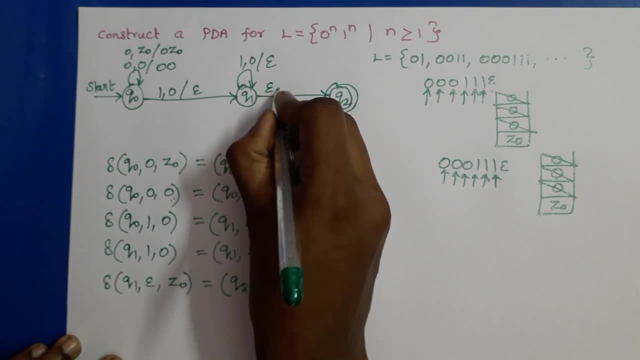 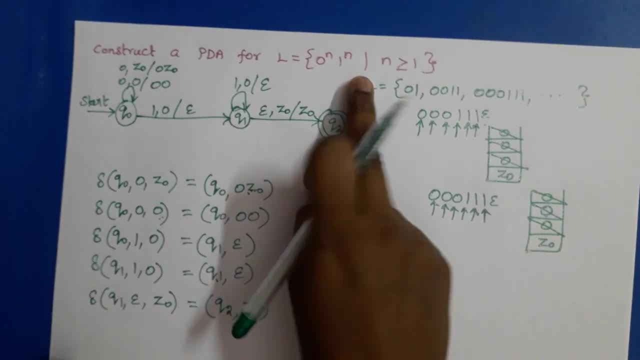 the edge should be labeled by epsilon comma: Z naught, slash Z naught. So this is a transition diagram for 0 to the power n, 1 to the power n. Now we can say that our input string has n number of 0's. 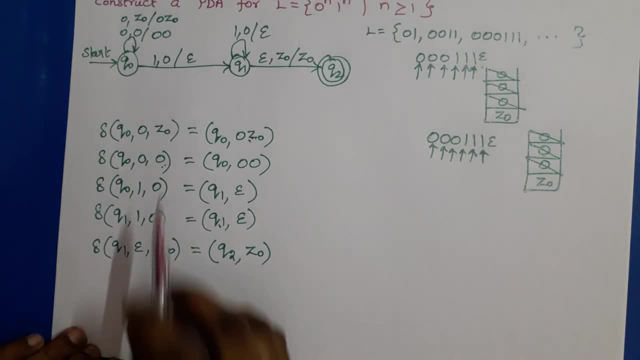 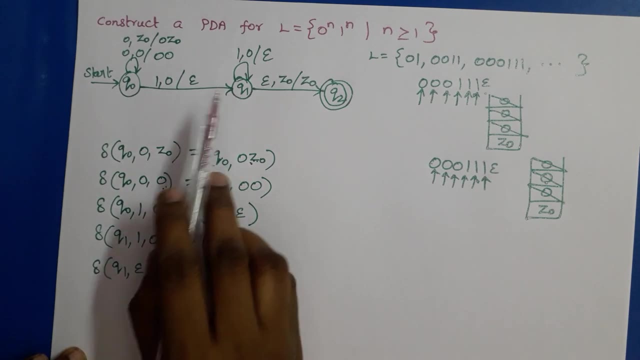 0's followed by n number of 1's. And here to perform pop operation, we need to change our state from Q0 to Q1.. Because if you don't change our state from Q0 to Q1, that is, if you want to perform pop operation also here. 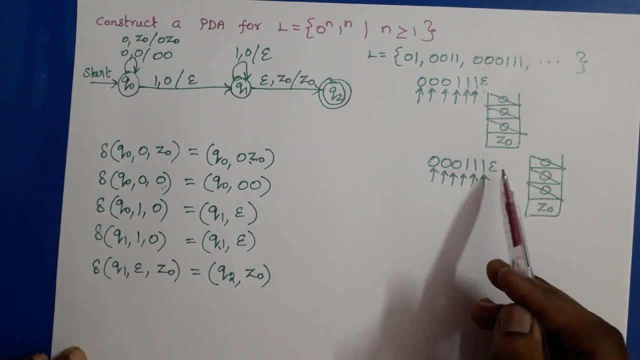 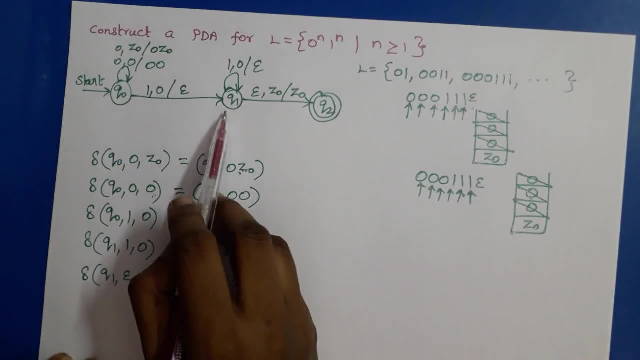 means then after 1. also, if some number of 0's will come, then that will also be pushed onto the stack Right. So we have to change our state to next state, Then only number of 0's. 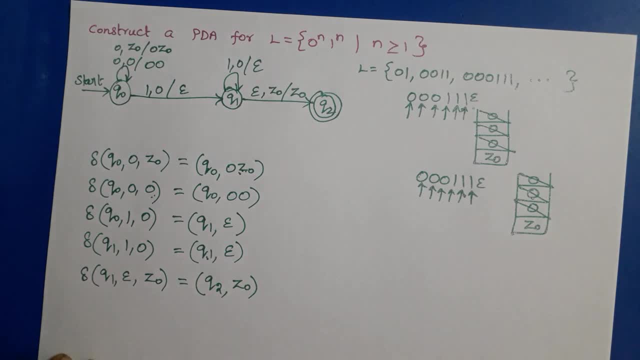 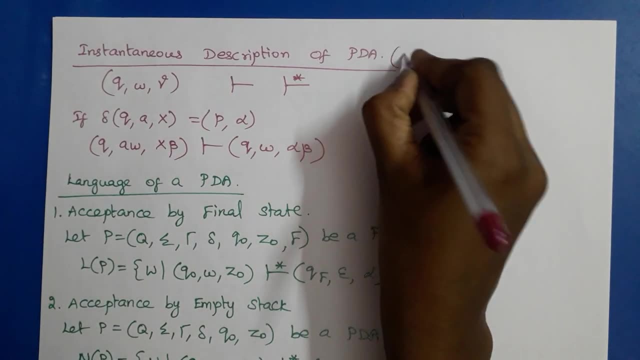 0's must be followed by number of 1's. After 1's, no 0 will come. Next one is instantaneous description of a PDA or moves of a PDA. Instantaneous description, or we can say ID, of a PDA. 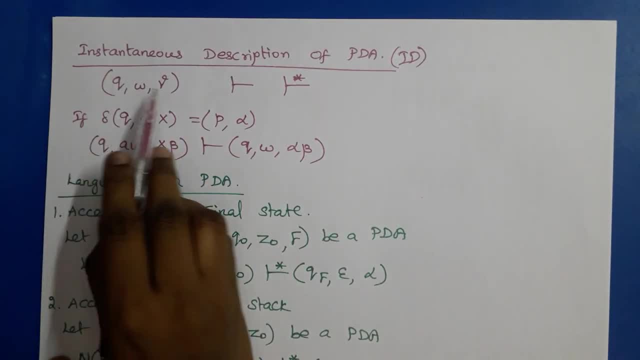 So it is represented by a triple Q, W, gamma. Where Q is a current state, W is a input string and gamma is a stack content. It may be a string. Okay, So these two are the string And it is. 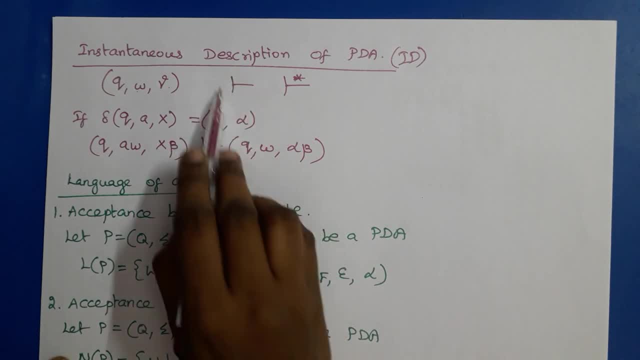 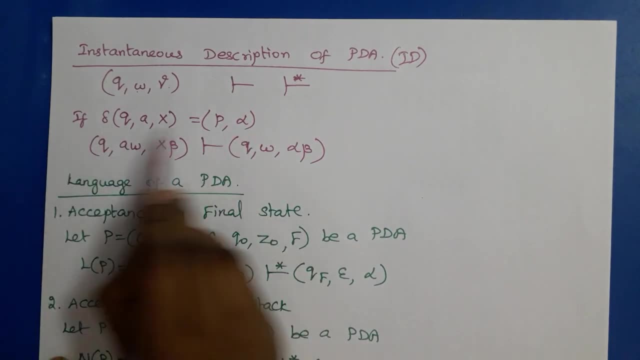 normally represented by the turnstile notation. So it represents 1 move and star means it represents more than 1 move. Then if a transition function, if a PDA, has a delta like this, that is, delta of Q, A, X equals P, alpha. 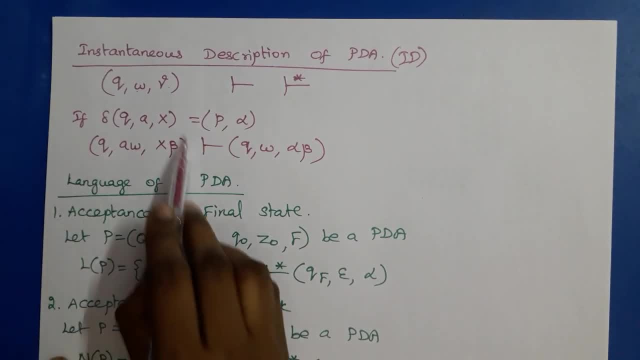 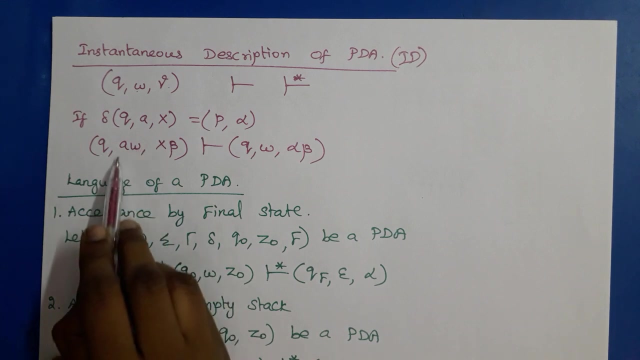 then the current configuration of a PDA is this: one means Q, A, W. The thing is: A is the current input and W Q means it may be any input string. So A followed by some input symbols. The thing is. 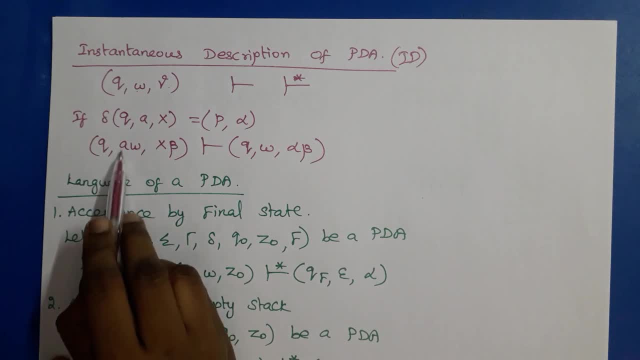 input pointer is now pointing to A. That is finite, control is pointing to A And top of the stack is X. Then other stack symbols. Okay, X is on the top, followed by some other symbols. So left end of the string represents top of the stack. 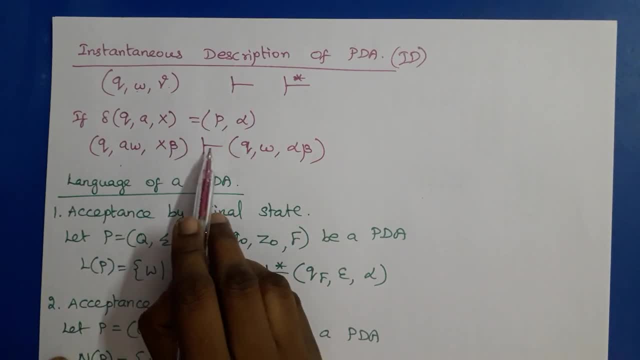 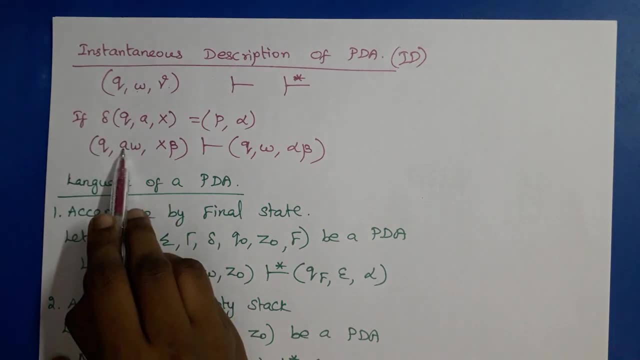 Means. then write the turnstile notation here. That is in one move how it will be changed. Q is the current state. Top of the- sorry- current input symbol is A and top of the stack is X. Then 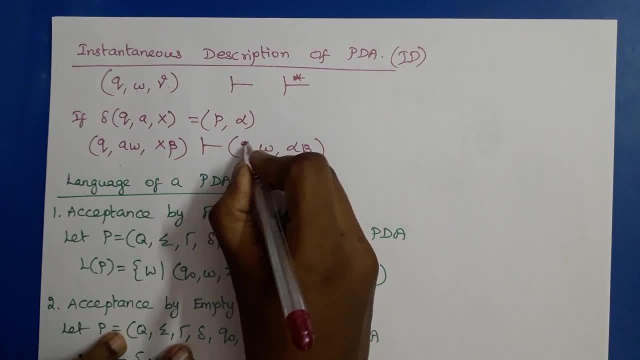 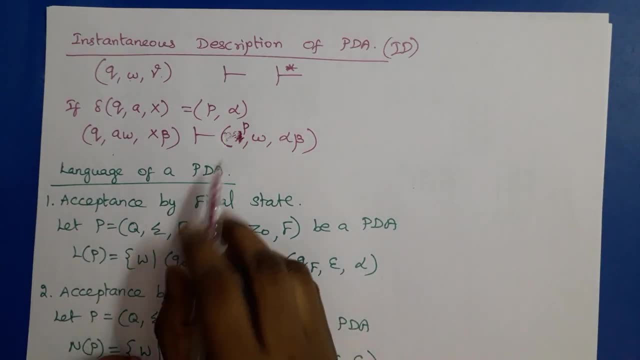 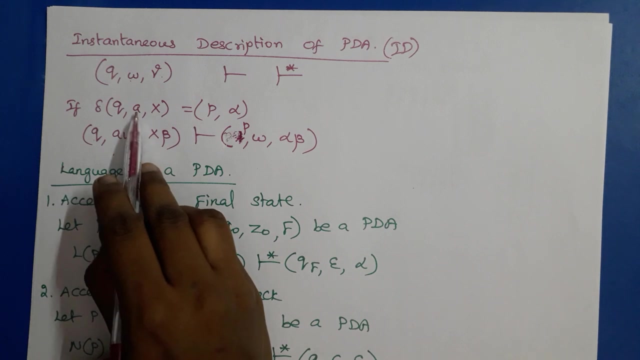 it goes to the new state P, So sorry, here P should be written P and sorry here. next state is P, So Q. Q changed to P, So P should be written here. A is the input symbol. 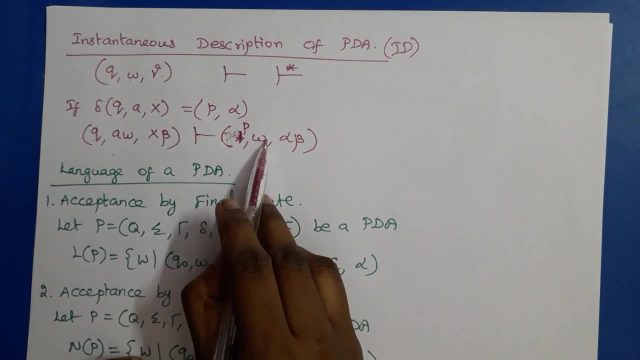 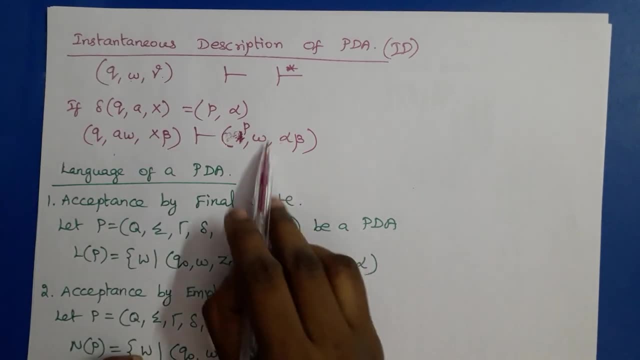 means it is consumed. So we have to write the, the remaining string, So W alone should be written. Then X is X must be replaced by the string alpha, So X is replaced by alpha, then followed by beta. 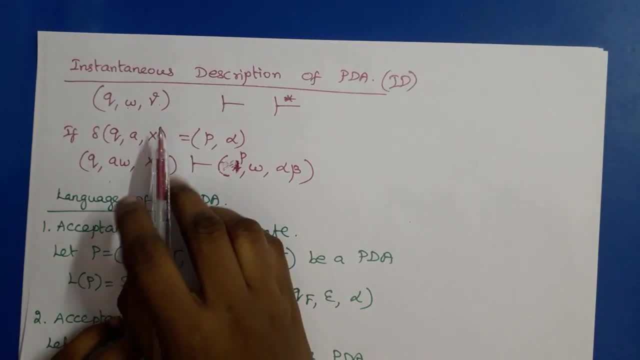 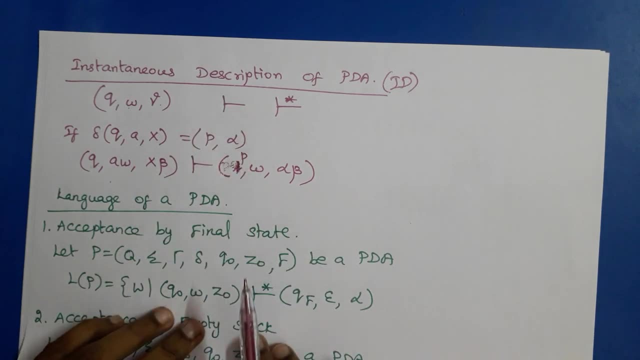 That we need to write. So, with the help of, with the help of information- sorry, instantaneous description- we can check whether the input string is correct input string or not. So consider the same example: We need to check whether 0011. 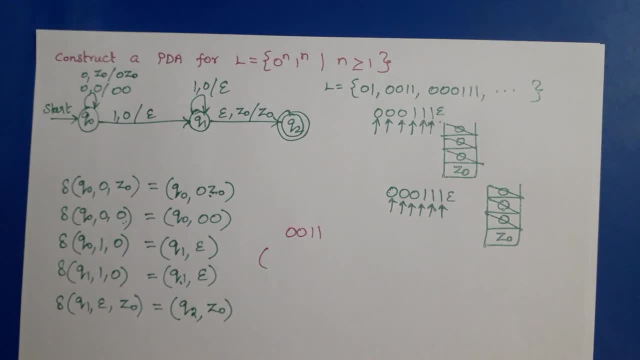 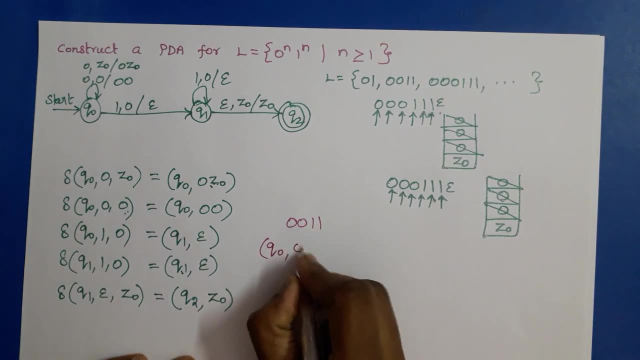 is accepted by our PDA or not. So we have to use the instantaneous description. So we have to start with the start state Q naught and write the input string W. We have to write the input string 0011 and initially, 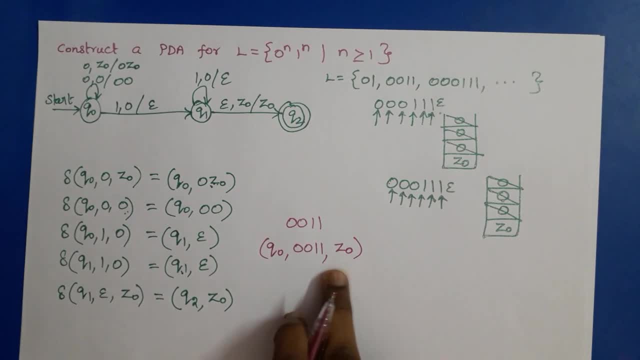 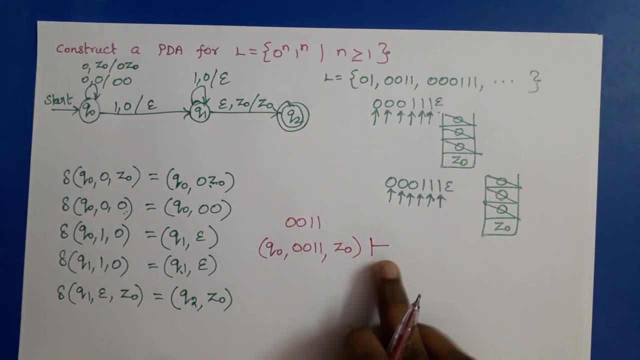 stack content is Z naught. right. Z naught will be on the bottom of the stack- top of the stack initially, So it indicates bottom of the stack. So we have to write the tangential notation here and by following the transitions. 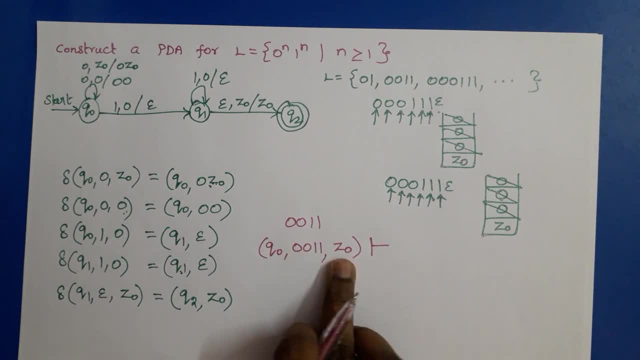 we can make the moves here. So Q naught 0 Z naught. Q naught 0 Z naught. delta of Q naught 0 Z naught means we have to follow this, So the next state is Q naught. 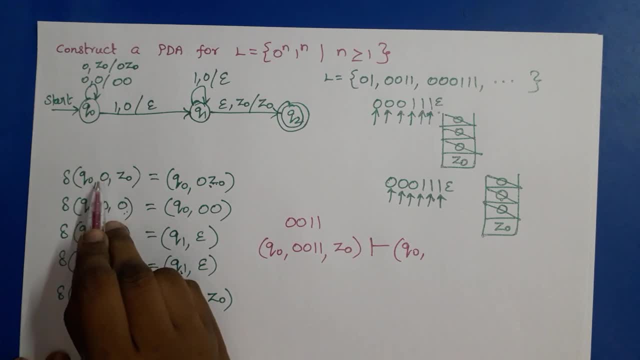 and 0 is considered here. So if epsilon is given here, then we should not remove that input symbol from the input string, But symbol in the sigma is considered. that is, input symbol is given here, then we have to remove that input symbol from the string. 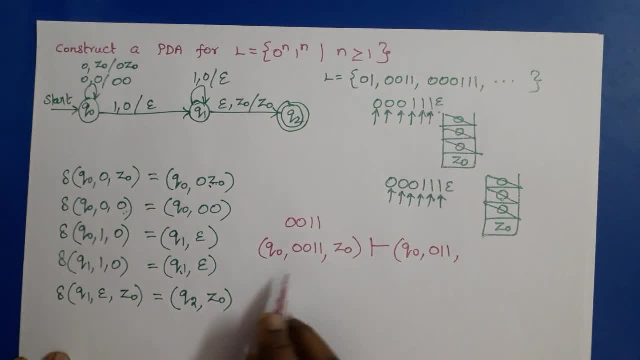 So the remaining input string is 011.. Okay, because here 0 is given, Then Z naught. Z naught should be replaced by 0 Z naught. So this Z naught is replaced by 0 Z naught. 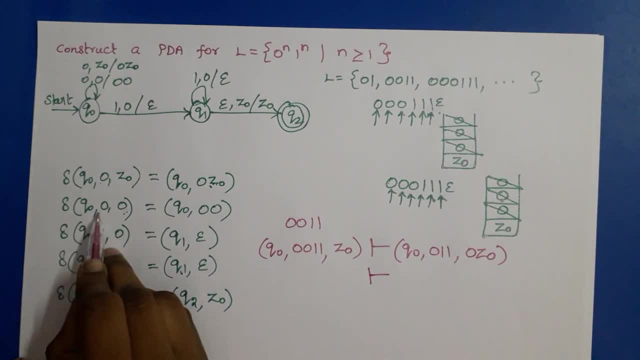 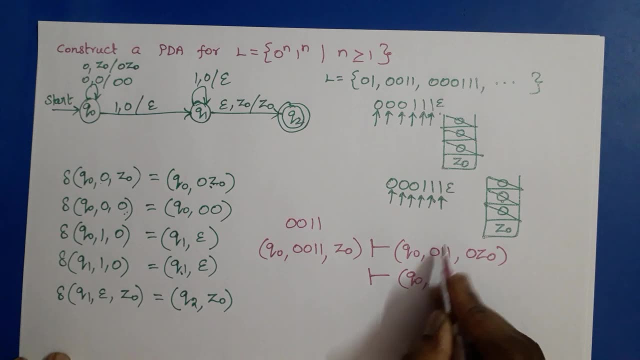 Now: Q naught 0: 0, Q naught 0: 0. So we have to follow this transition. The next state is Q naught Here. 0 is given, So remove 0 from the input input string. 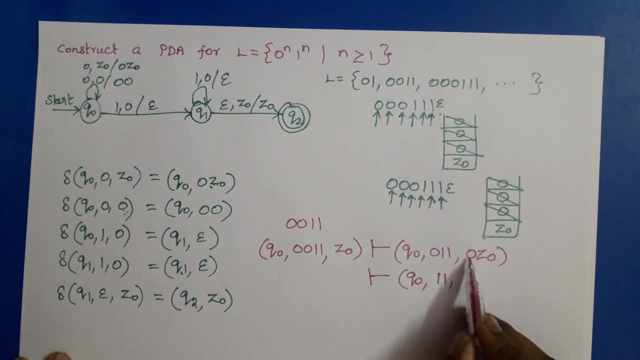 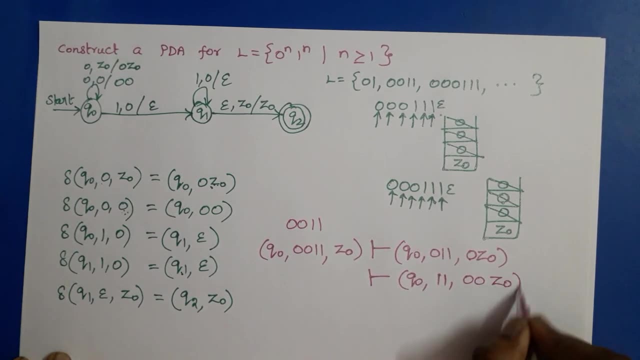 Then 0, the top of the stack, this 0.. Okay, this 0 is replaced by 0: 0.. This 0 is replaced by 0: 0.. No change in Z naught Now Q naught 1: 0.. 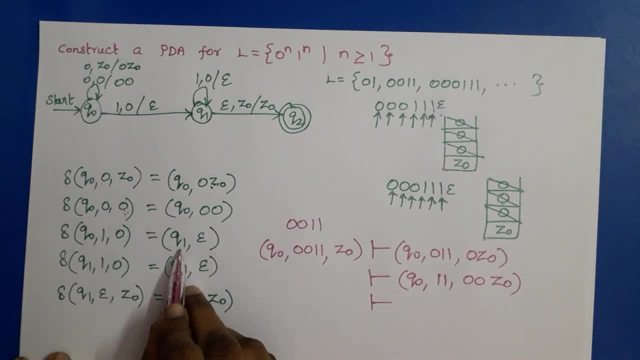 Q naught 1. 0 means the next state is Q 1.. 1 is given here. that is input symbol. So remove 1 from the input string And 0 is replaced by the top of the stack. 0 is replaced by epsilon. 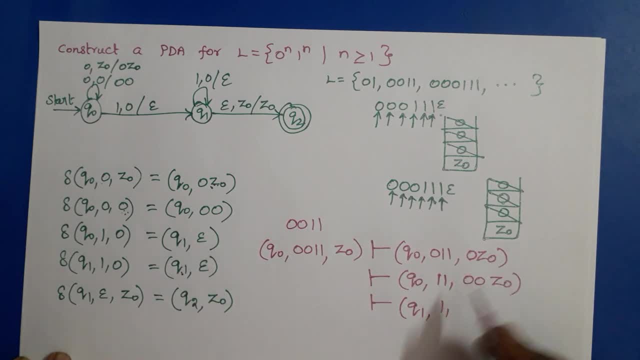 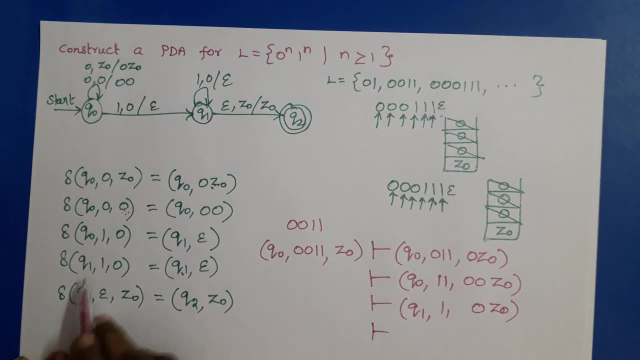 Epsilon means do not write anything, just remove this 0.. So 0 Z naught. The thing is, pop of the stack is performed. Then Q 1 1 0.. Q 1 1 0.. 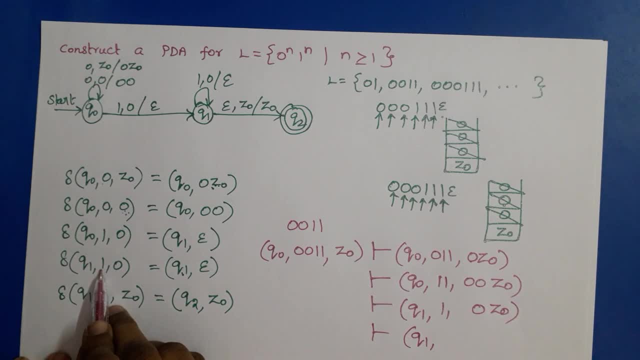 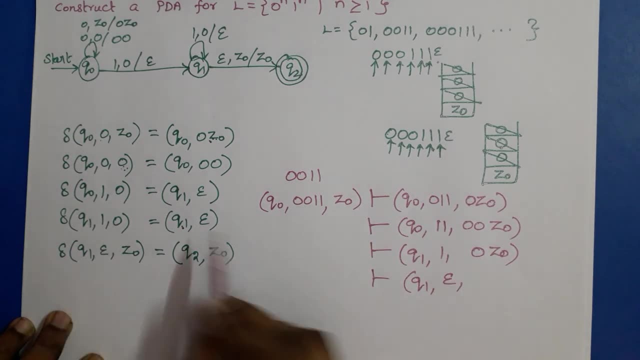 The next state is Q 1.. 1 is considered here, So it is removed. So the remaining symbol is epsilon. Then 0 is replaced by epsilon. Now Q 1, epsilon Z naught. So Q 1, epsilon Z naught means 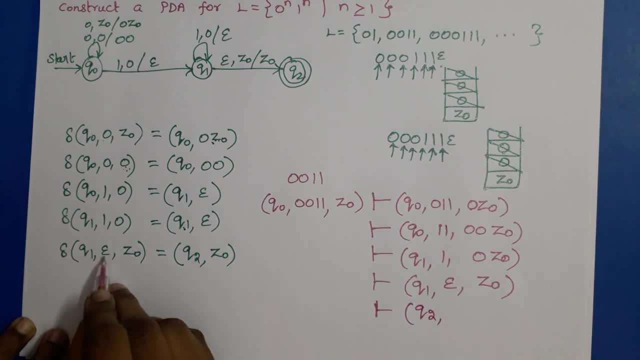 Q 1. change to Q 2. Epsilon is given, So do not remove anything. So still it is epsilon. Then Z naught is replaced by Z naught. So now there are two types of languages. 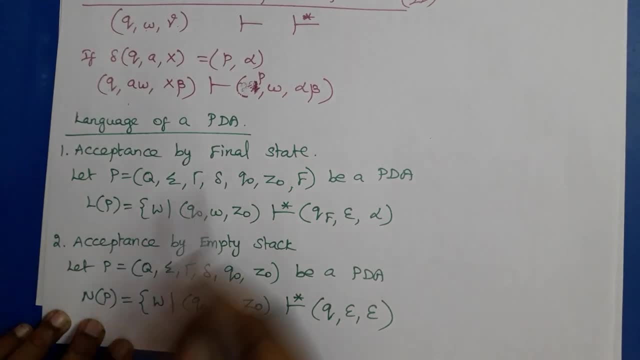 Languages of a PDA. In two ways we can say the language of a PDA. There are two cases: Acceptance by final state, acceptance by empty stack. So let PDA is a 7-tipule notation, Then L of P is equal to. 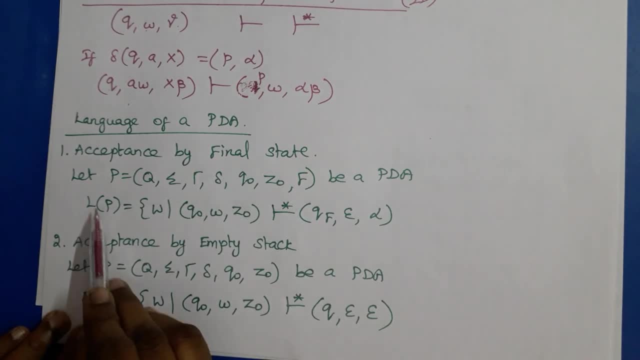 L of P Language acceptance by final state is represented by L of P- is equal to set of strings W, such that, that is, these set of strings are belonging to this language if it satisfies this condition, That is, if we start. 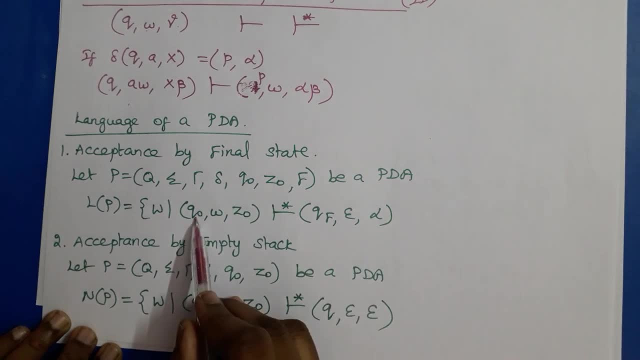 doing the instantaneous description with the start state Q naught and the input string W and the starting stack symbol Z naught in some number of moves. if we reach Q F, Q F means it is a final state. Okay. 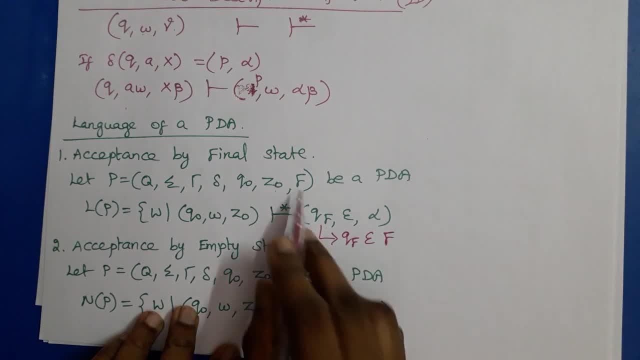 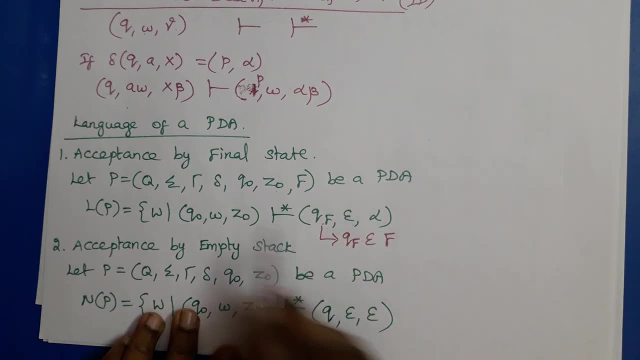 It belongs to Q. F belongs to F Means if we reach the final state and the input symbol is fully consumed. But the stack content may be anything Means we can say that the language, the string is accepted by our PDA. 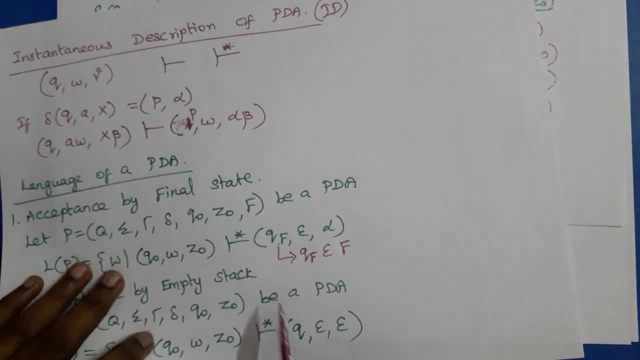 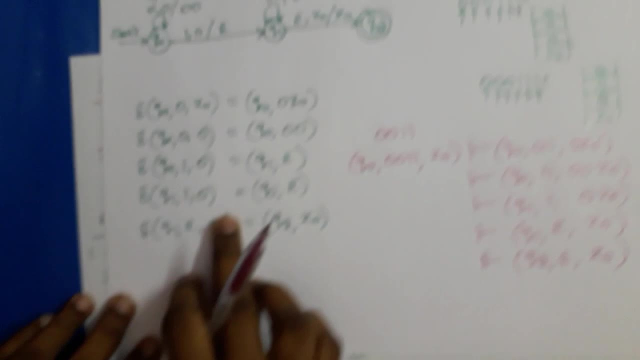 So in this example we reach the here Q F Right Here Q 2 is a final state. So after, after constructing the set of transition functions, we have to write the 7-tipule notation also. So PDA P is equal to. 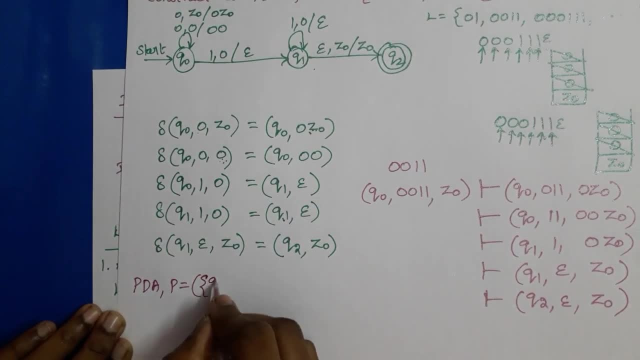 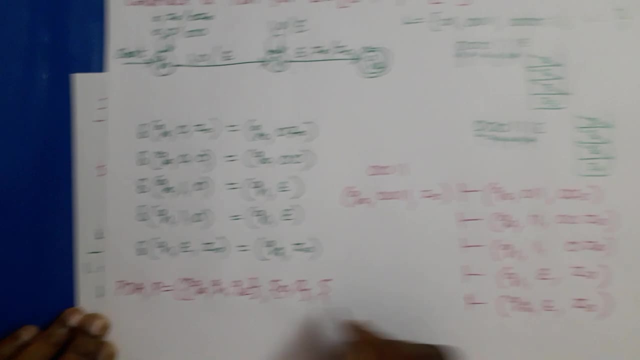 the set of states: Q naught, Q 1, Q 2.. Input symbols: 0s and 1s. Stack symbols: in the stack we will push only Z naught and 0. Right, So 0 comma Z naught. 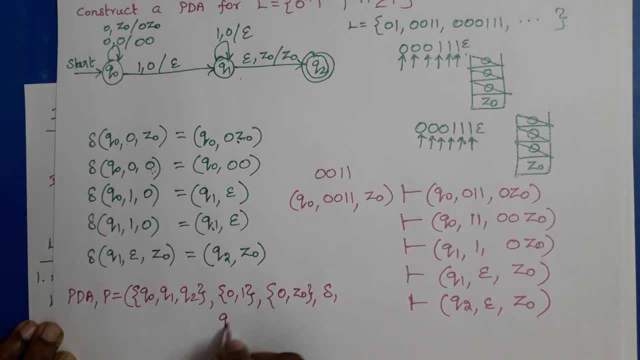 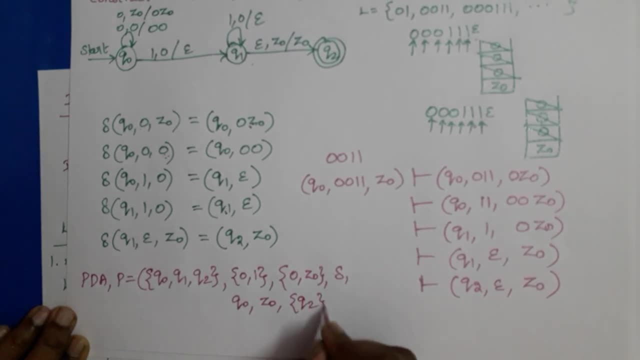 Delta is a transition that we have written. Q naught is a current state, Z naught is a starting stack symbol And Q 2 is a final state. Right Q 2 is a final state. So in this example, 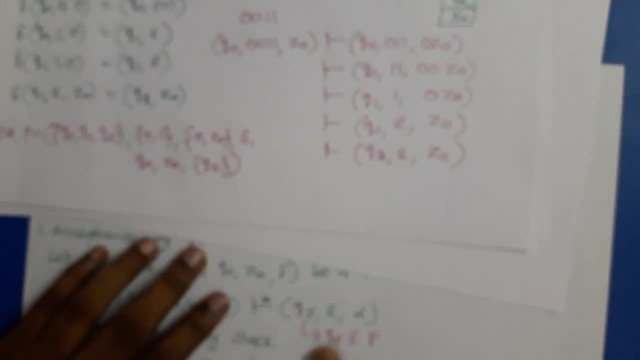 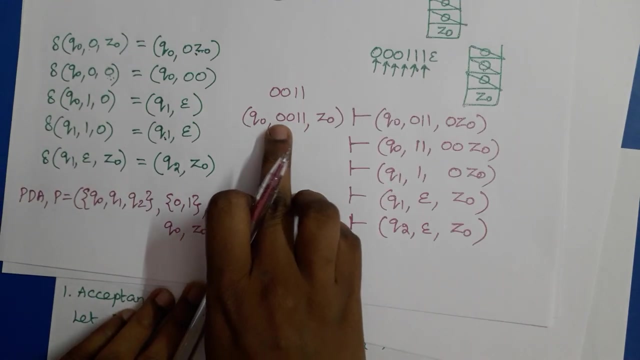 we reach the final state, Q, 2.. And the input string is emptied, Okay, And the stack content is anything. So we can say that 0, 0, 1, 1 is accepted by this PDA, And we have constructed this PDA by. 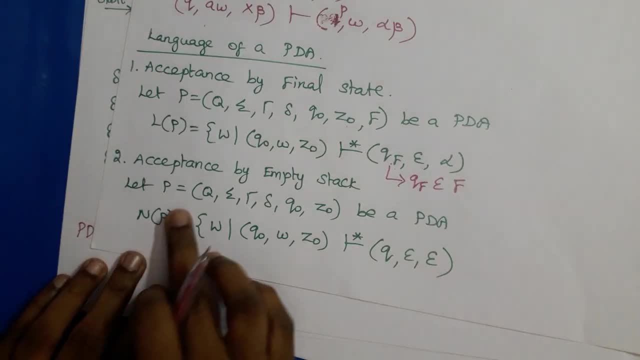 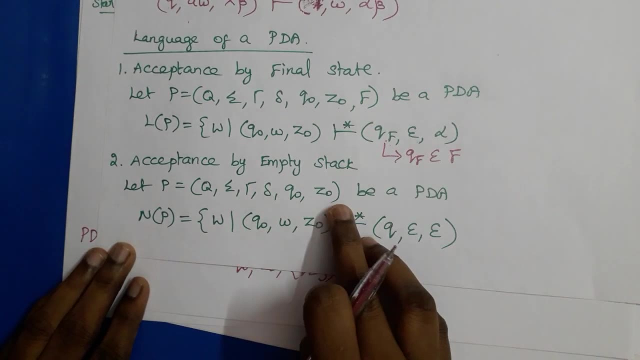 final state. Another one is acceptance by empty stack. So here let PDA. P is equal to Q, sigma, gamma, delta, Q naught, Z, naught. There is no need to mention about the final state, Because this is acceptance by empty stack. 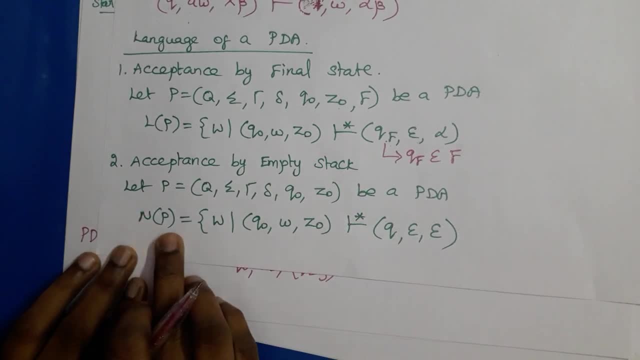 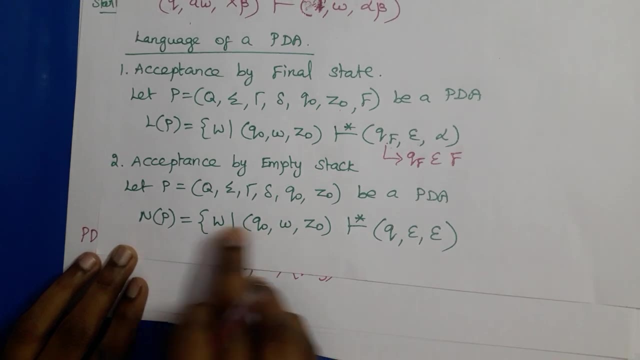 So it is represented by N of P is equal to set of strings W, such that we have to write the same Start state: Q naught, W, Z naught. In some number of steps it may be any state. 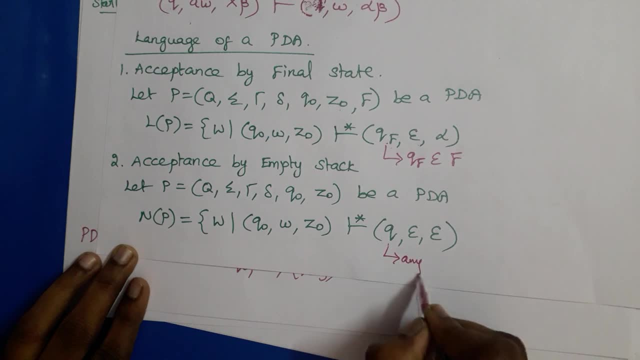 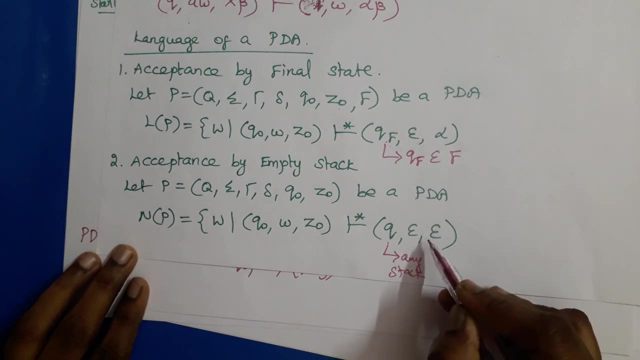 Okay, No worry about the state, But the input string should be fully consumed And we have to empty the stack. So here, final state and empty the stack. So here, final state and empty the stack.